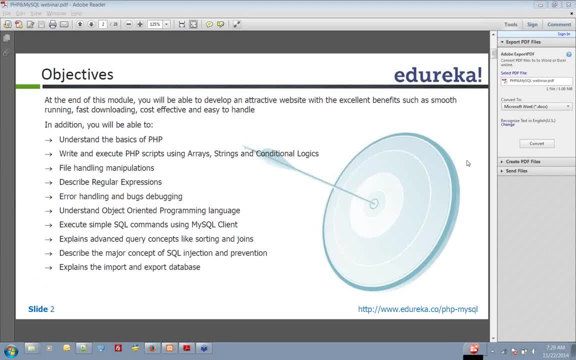 Understand the basics of BSP writing small BSP programs, so understanding the control statements, arrays, strings, variables. how to handle files, how to use the regular expressions, error handling and debugging, executing MySQL commands, query concepts and the security issues which are related to SQL injection and prevention. how to protect your. 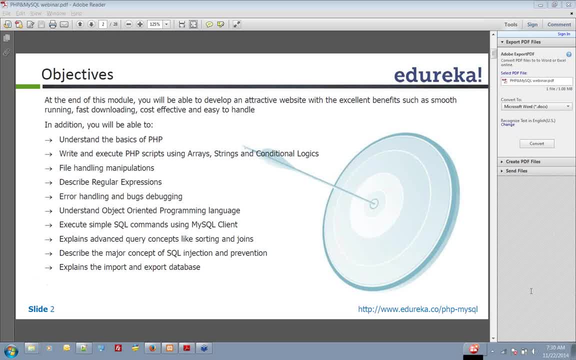 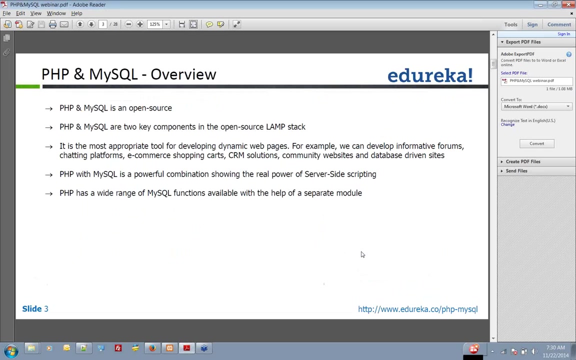 application from outside attacks. how to import and export your database from one server to another server, from one machine to another machine. Okay, so that is the objective of this course, I hope, since you are from a programming background, so you understand the basics, or you may have. 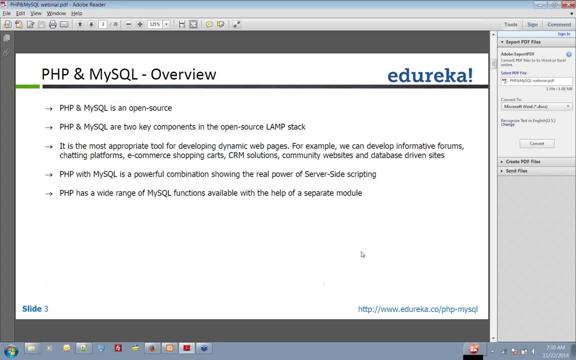 somewhat knowledge on this technology: BSP and MySQL. So both are open source, BSP and MySQL. So since it's open source, it's really available. You can download and install. And these two are the part of LAMP, LAMP stack. LAMP stack is nothing but Linux, Apache, MySQL and PHP. So when you say LAMP, 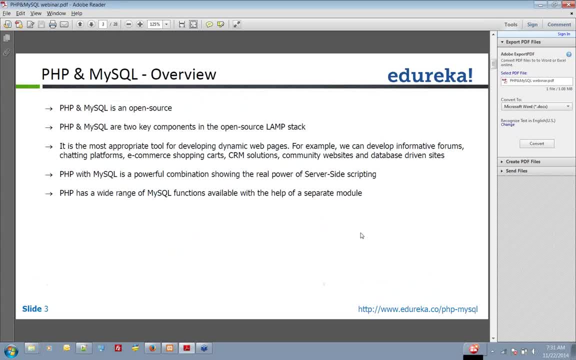 stack. it does mean that it's a PHP MySQL along with Apache, So sorry. So what is PHP? So PHP takes a lot of information. It takes a lot of information. PHP is like server-side scripting language. It is loosely coupled, So by this you understand. 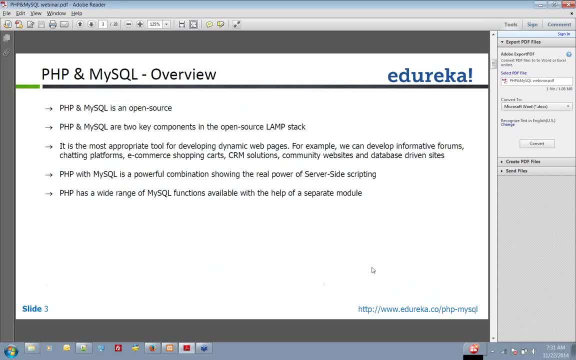 what it means by loosely coupled. But in PHP there is a little difference where variable declaration varies. In PHP we don't need to define the variables explicitly. The value whichever you will assign to a variable, the variable will be assigned to the variable. 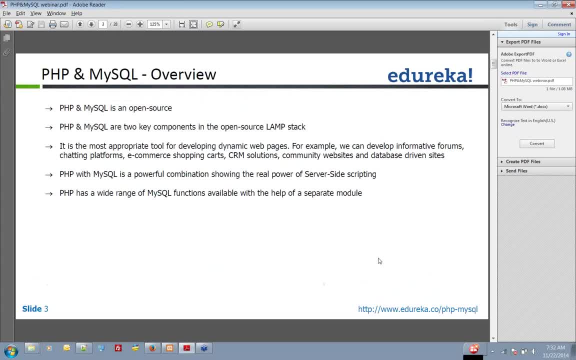 The variable will take that form. What does that mean? So suppose, if you assign a string to a PHP variable, that variable becomes string. If you assign integer, that variable becomes integer. So there's no need to define that variable explicitly, Just like in other languages. 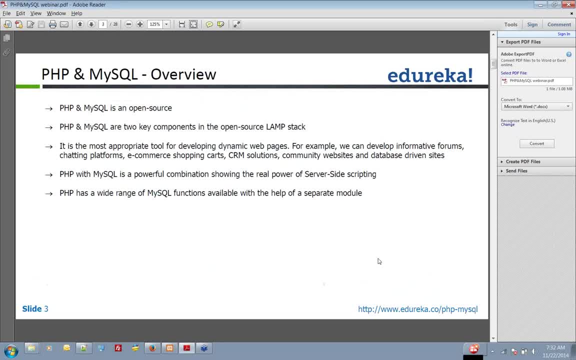 C, C++ or Java, where you define string and the variable name, integer and the variable name. So that is not required. So that is what this loosely coupled is. Now, what is server-side scripting language? So server-side means it runs on server In. 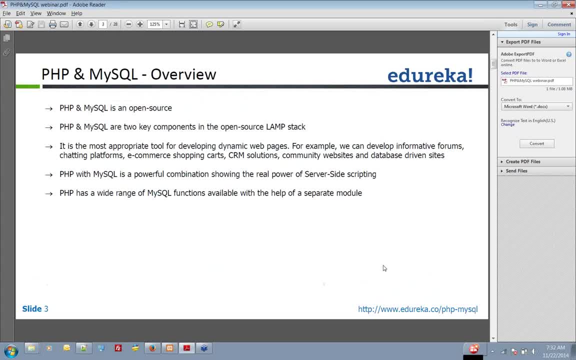 PHP. you must have seen on the websites we are exploring on the browser. The browser interprets the HTML tags, but it don't process PHP, because the long form of PHP itself says PHP is a PHP hypertext processing. Now what do you mean by pre-processing, Since PHP runs on a server, so whenever there 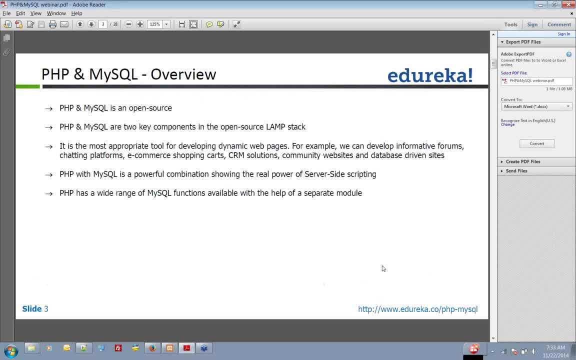 is a request for a page, and if that page has PHP, then first it will run on the PHP server. It creates that HTML output and sends back to the browser, And browser displays the plain HTML part only. So that is what is called a server-side scripting language. 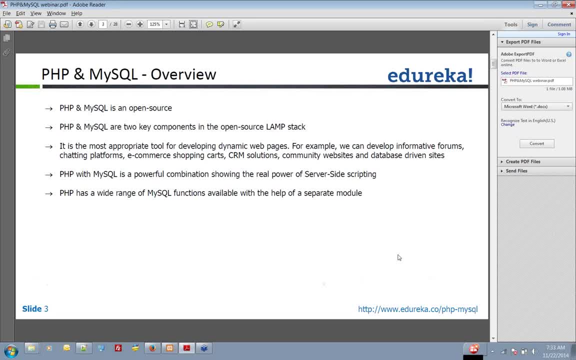 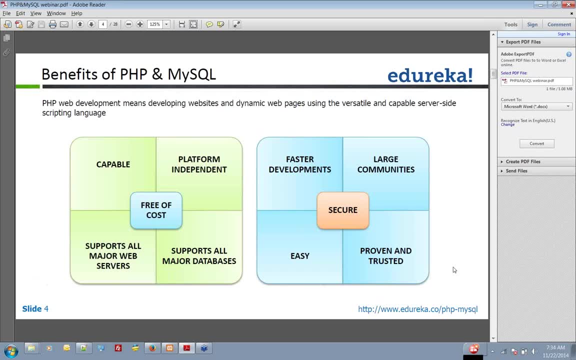 And it is so powerful that you can develop anything. Now the benefits of PHP Benefit is like PHP and MySQL always comes together, But it is not platform-independent or the database-independent. So you can run it on a server but you cannot. run it on a browser. 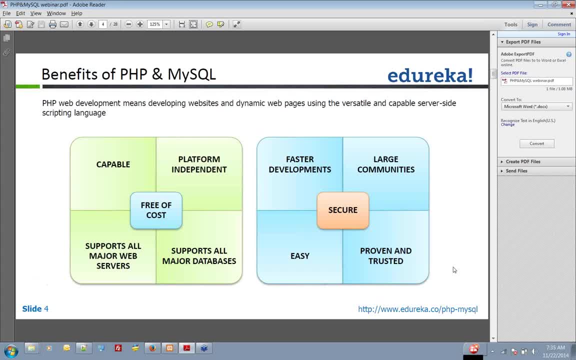 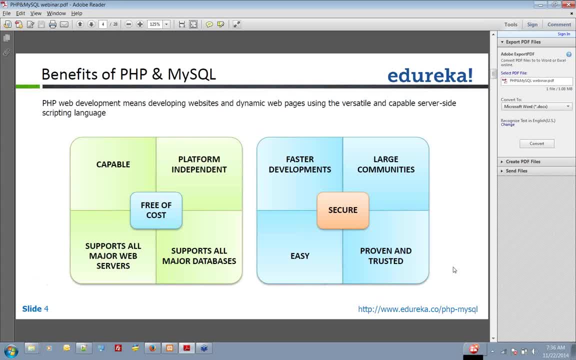 But if you are writing vanilla PHP, so you need to take care of the security issues And it's more easy to understand proven and trusted technology, PHP, MySQL. You must have seen many websites developed into PHP, even like Facebook, India Times. 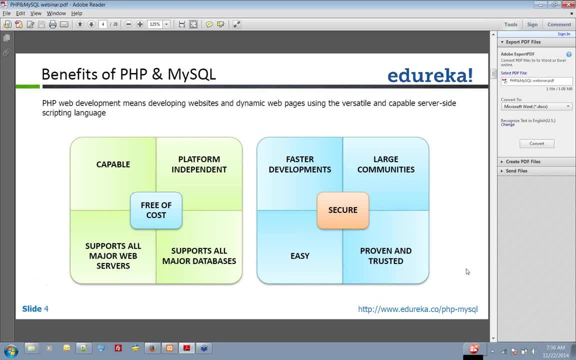 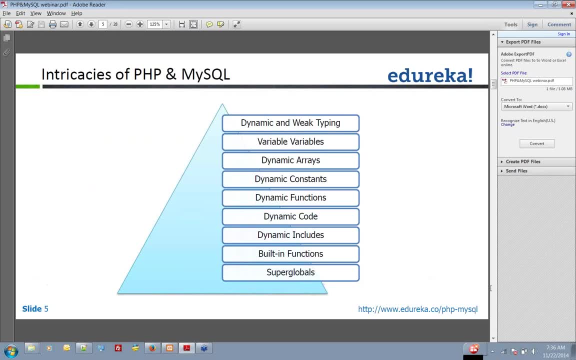 Reddit. There are a lot of good websites, So, as I said, weak typing- that means variable declarations- is not required. One more new thing introduced in PHP is variable variables. You must have heard this word the first time, But variable variables. 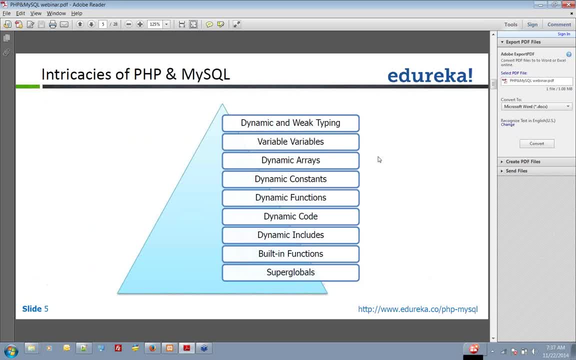 Variable variables are like the changing form of the variable. When you assign a value to a variable, that becomes like variable value. But in PHP you can assign value to a value, So that is called variable variables. Suppose you have a variable A and you assign a value B, So your B can also be a variable. 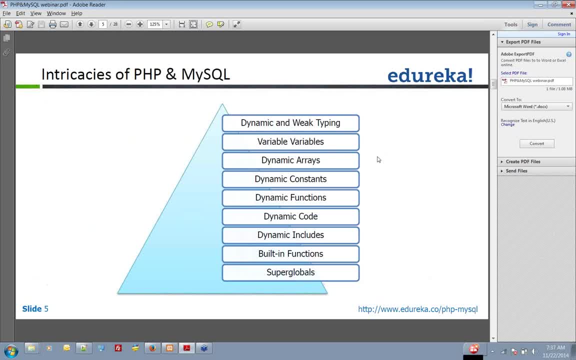 You can assign a value to B. So that is one more thing, Thank you. Thank you very much, Okay, Thank you. 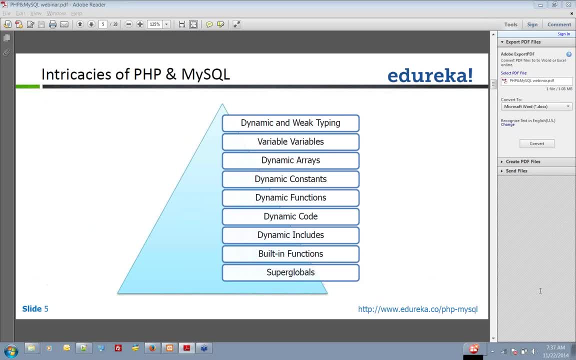 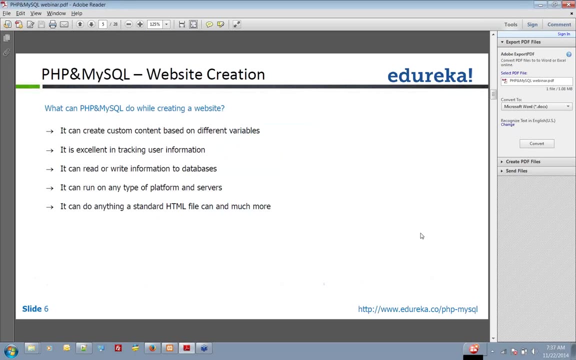 You know, go for javanet. that depends on the platform and the application they're developing. So we'll come to the question and answer in the later part of this session. okay, Okay now. creating a website in PHP. 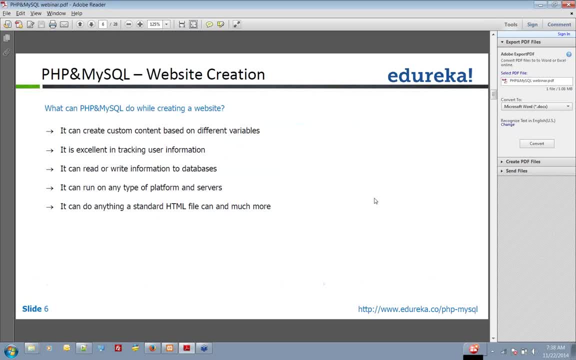 So in PHP we have, like the variable are different types of variable we have here. also in PHP We can make use of those variables to you know. maintain the user information also in the forms of cookies sessions, which is in terms of like tracking user information rewrite. 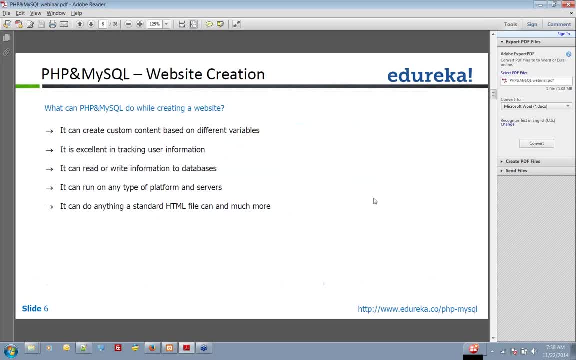 information from database, That is, the database connectivity claim. Okay, So we have, like this, a lot of transformative changes And there are not any type of platform or server. Like I said, it can run on Windows OS. also, It can run on Linux and the different web servers. 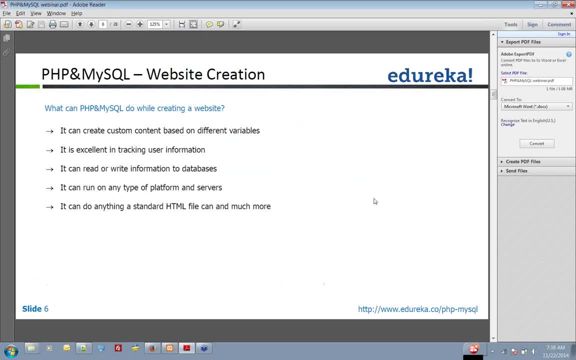 You can configure it on iOS web servers also and the Apache web servers also By default. from start, we came with Apache web server because it was the most compatible server. It was considered earlier. Okay, It can do anything a standard HTML file can do, and even much more, since it's a dynamic. 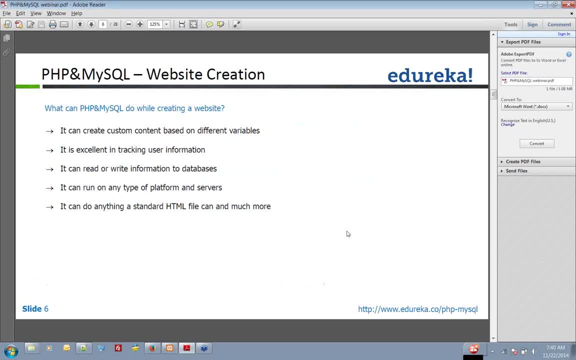 language. Let me tell you about the PHP history a little bit. When PHP started, it was not called PHP- The actual name is Personal Home Pages, which was written by. the first version of PHP was written by Rasmus Lethoff, who is called the father of PHP, and when he developed it he 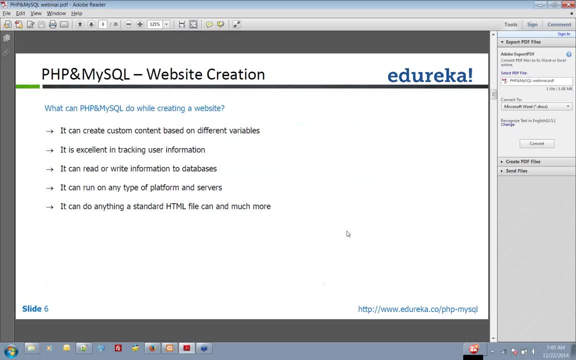 developed it for writing his own resume and to keep it online and to access. After that, two developers like Zeb Swarovski and Andrew Gutman, they rewrite the core of the PHP and they came up with an engine called Zen. So Zen is the combination of two names: Zeb and Rasmus Swarovski. 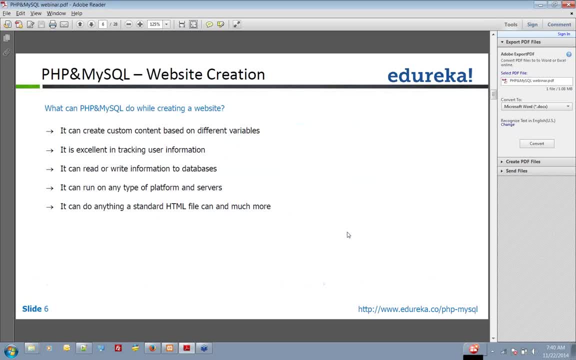 So that was the combination of two names and it was called Zen engine. After that they came up with 3.0 and then the next version of PHP was 4, where they have added a few features, which was supporting object oriented cards. So in the last release of PHP this was PHP 5.3, they have added full support, even it. 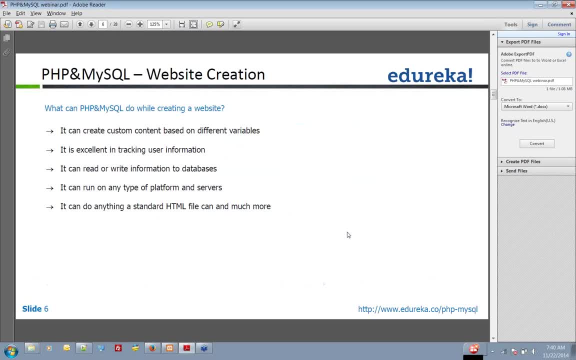 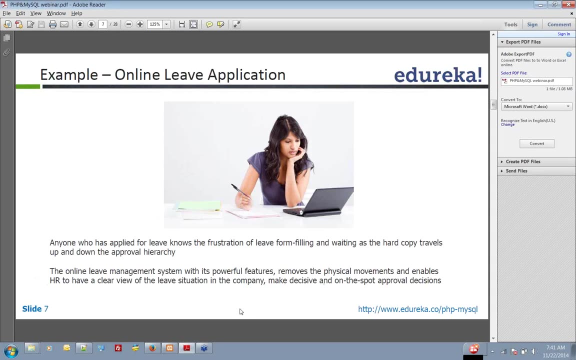 was added into PHP 5.2 also, and the latest version has almost all the features supported, and So that was the little history on PHP. Okay, In this session we'll be, we'll be Okay, We'll be looking on to one real life situation like online application where you can understand. 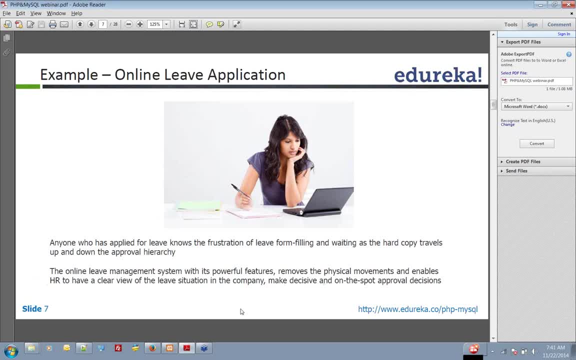 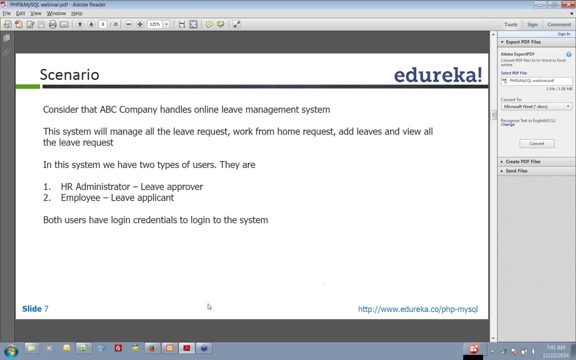 the use of PHP, how to write the code, how to execute it. With this example you will understand it better. So online application is like all of us must have used. So it's a request and response model where you request for a leave and you request for. 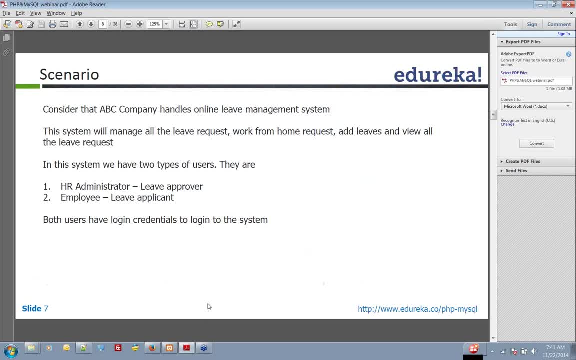 a leave And the response is accept or reject from the HR department. Now here is a scenario to consider that company ABC handles online leave management system. The system will manage all the leave request, work from home request add leaves and view all the leave request. 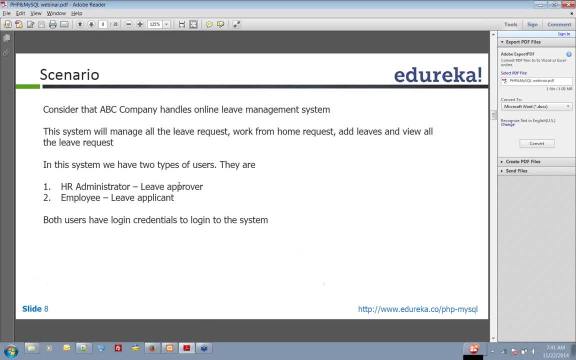 In this example you can see that the system will manage all the leave request, work from home request and view all the leave request. The problem over here will be that when they are supplying all of the leave request, they did not manage all of the leave request and how they expected the leave and leave didn't. 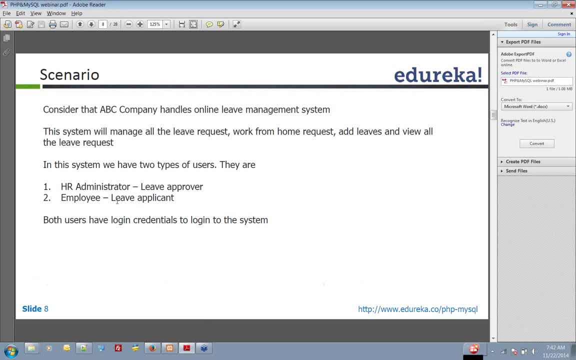 change the system or not. So they have never working properly with the creating of the Chunjooence tengas, because there's no matter. you set up an AB device on the dejar And with the help of the working systems, they are successfully inside the system. 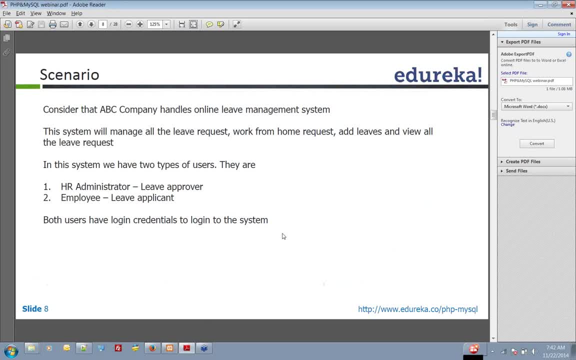 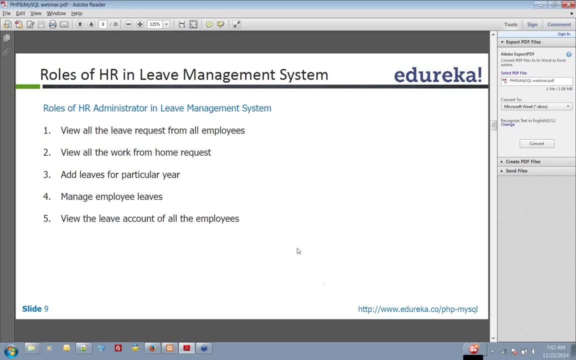 Okay, and they will perform their own task. Employee will log in and he'll send a leave request and the HR administrator will check all the leaves applied and will approve or reject. So, as I said, HR administrator can see all the request came from all the employees. View. 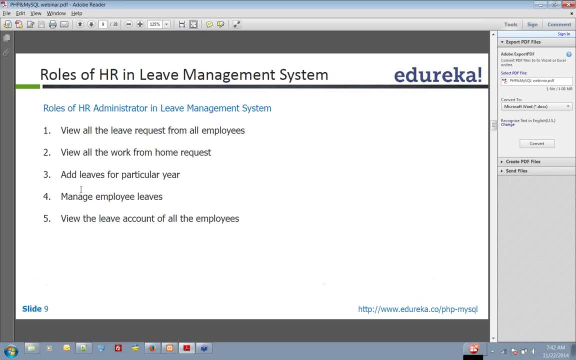 all work from home. request is the same as leave application. Add leaves for particular year, manage employee leaves. view the leave about all the employees. So this is the system we'll see in actual running. So this was the role of HR administrator, Now the employee. 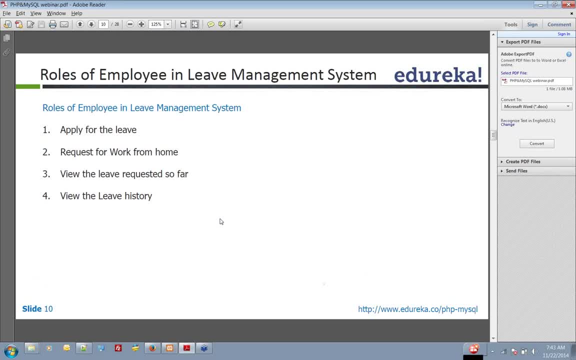 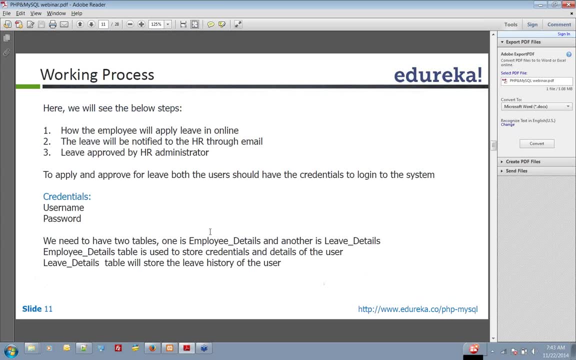 what employee is the HR administrator? What is the role of the HR administrator? What employee can perform is apply for leave. request for work from home. view the leave requested so far and the leave history. Okay, the working process, Since you are well aware of the working. 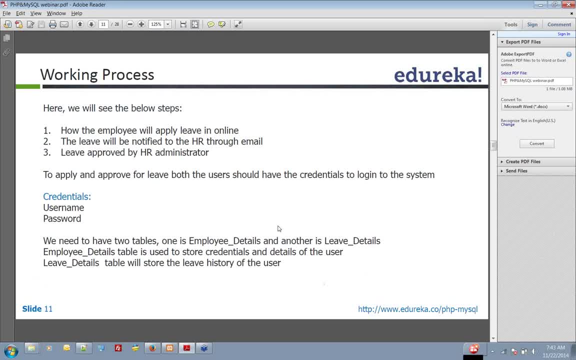 the online system of leave application. I will take you to the application page and the code so that you'll understand it in more details. Before that, I'm going to show you how to apply for leave- If that's supposed to apply- and approve for leave both users. 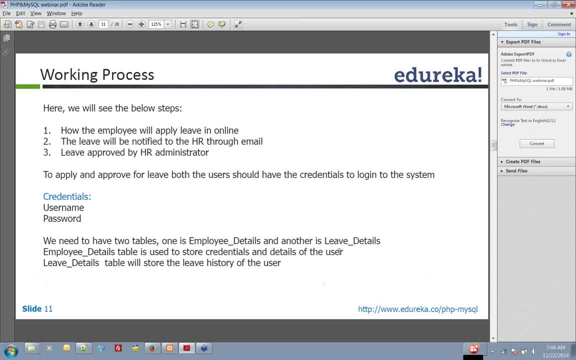 should have the credentials to log in the system. Okay, so we need two tables, which is one, leave details, the other is employee details, where we have the employee login information and leave details will have all the leaves applied, along with the status. So this is. 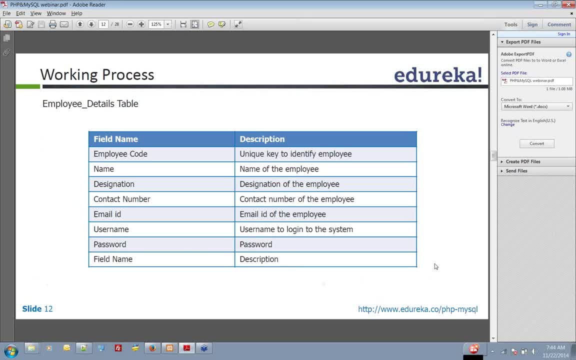 the employee table we have designed. So this is the employee table we have designed and the leave details table For this example. employee code, which is the unique key for the employee across the organization. name of the employee: designation contact number. 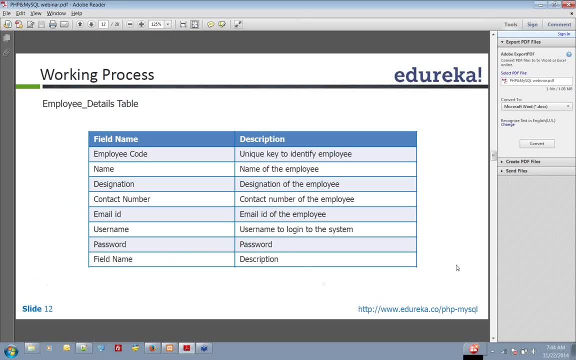 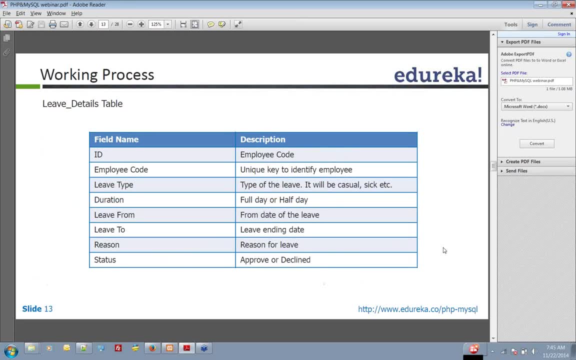 email ID, user name and password. These are the login credentials we'll be using And the leave details table. So this is just a generalized example just to explain you how to work with PHP and MySQL, How to connect it to database, how the application submits the data, how the application displays. 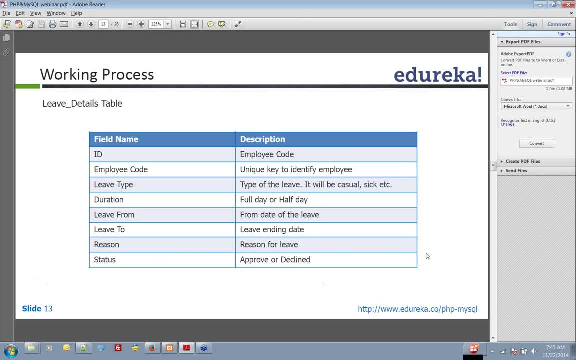 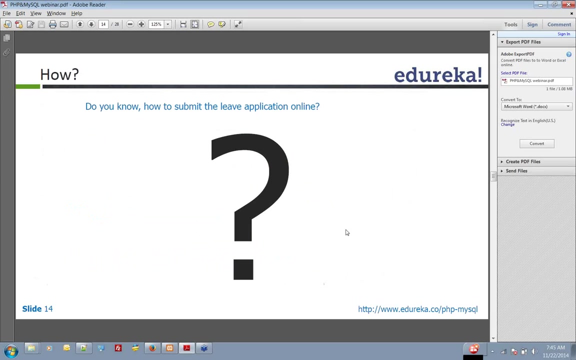 it. So this is just for the basic understanding. So the example is a little smaller. This table has duration leave, type leave from and to the region, along with the status Okay, now we need to have a. So I'm not sure like if your company has the online leave application. 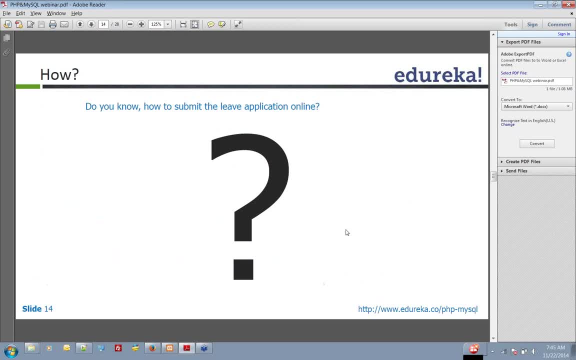 system, but the general procedure is to have the form to submit the leave application where you can enter all the form: date, two days, the type of the leave and the region. So I'll show you how This will be the form, Okay. 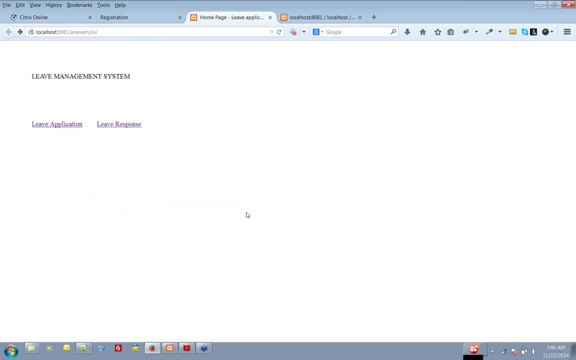 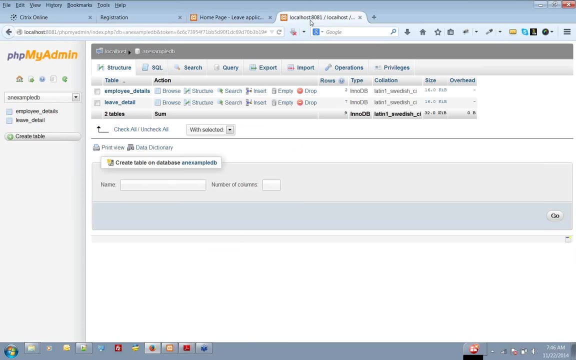 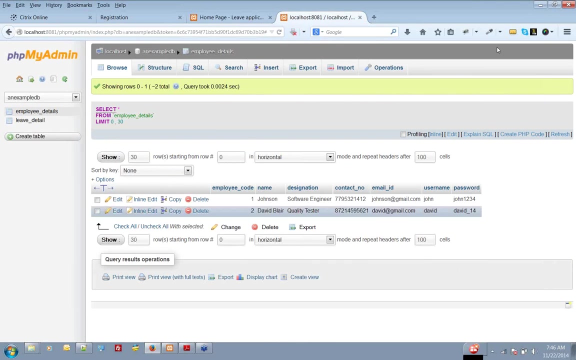 So consider this as a home page of this application, And you have already logged in. Since we are not, We have the user data here. Okay, so this is the employee table, And the interface you're seeing is phpMyAdmin. phpMyAdmin is like a SQL query browser where you can see: 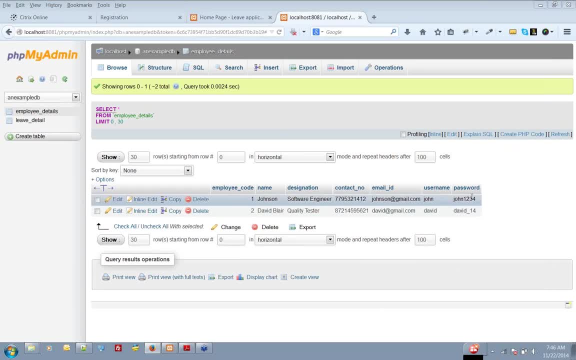 records of the data And it's free to use. So this is a kind of a database management system. So we have two tables created here with some sample data. This is the employee details table and leave details, All the fields which we see in this, I think in this example. 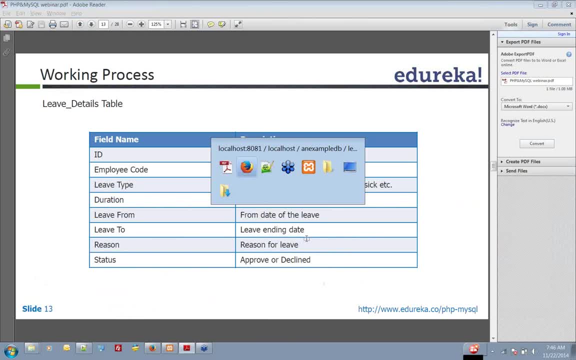 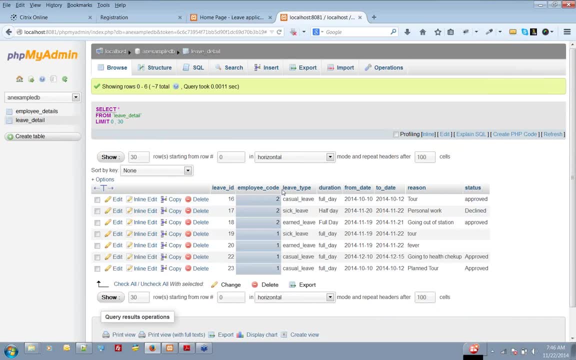 there are a few fields, so these are the fields. Okay, PDF are available in this table. Leave ID is the default key of this table. employee code, leave type, duration, season and state. So state will be updated by HR administrator and all these fields submitted by employees. 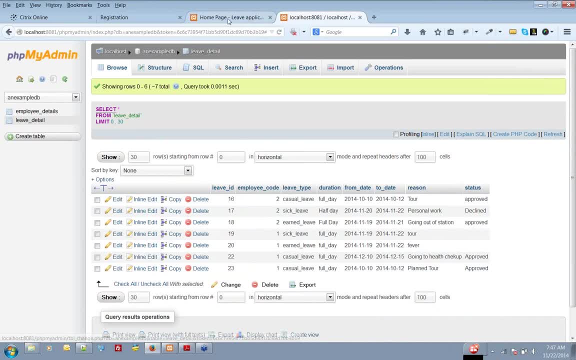 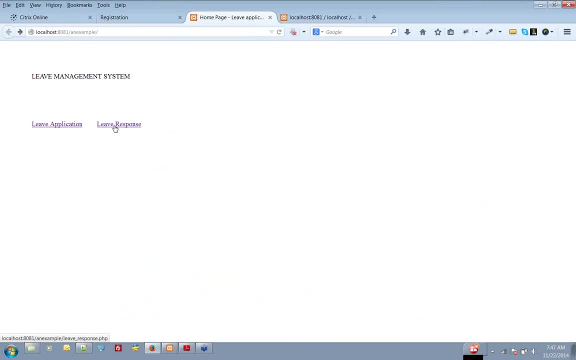 So how do the employees submit this? We have the leave application. this is the two URLs: leave application response. Leave response is for administrator, but since I wanted to show you the application, so I have combined both the URLs into one account. 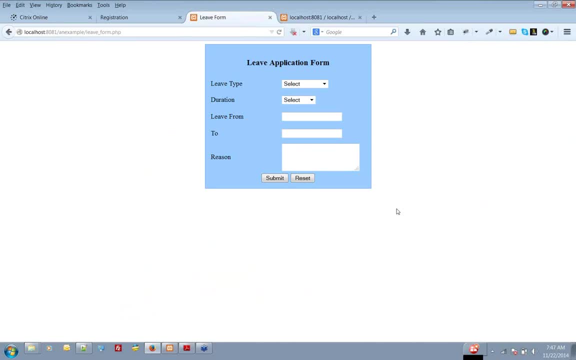 So this is leave application for the employee. Now we have fields like select drop down box. You can select the leave type, duration: full day or half day leave. from now this is the date. In normal practice every programmer should take care that if this is a date box, it should. 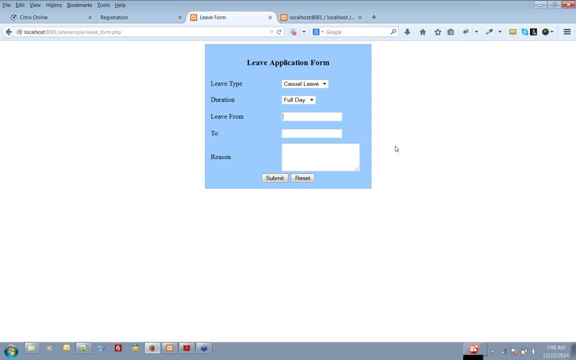 have the date ticker, otherwise it should have the date format mentioned so that the user can enter the date format. Since I know this format, so I'll enter it directly. Okay, now, here we are waiting for two dates. Let's consider some other date: 12 to 13.. 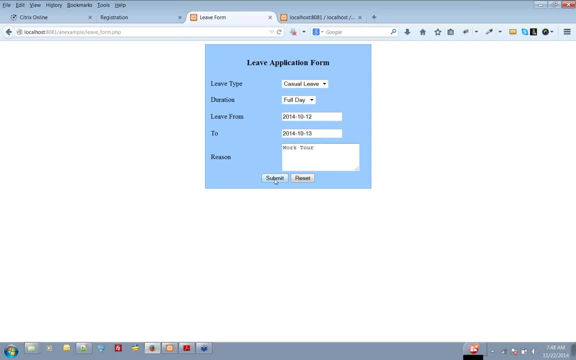 And we have one, two. Now we are submitting this application, So we should store the data into that table. Okay, So we are seeing this. Okay, So we are seeing this error. Whenever you came across such errors or warnings, just read carefully. as programmers, you should. 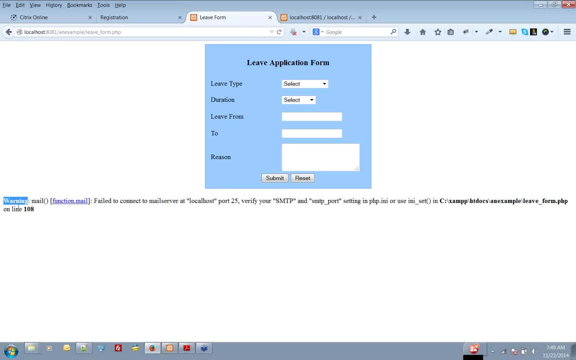 be focused on this, Like warning, or the warning means the application will stop. It will keep on executing, but still there is a warning that this function has failed to connect to mail server at local host. Now the problem with this is the SMTP server. simple mail transfer protocol is not configured. 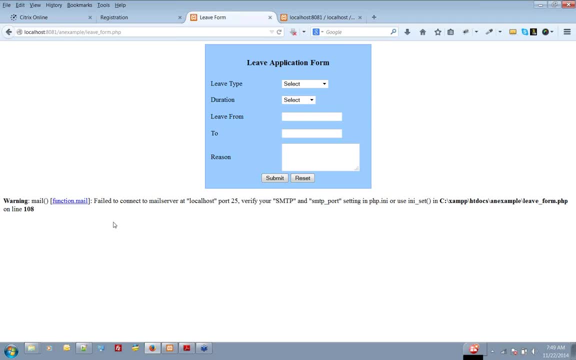 on this local machine, So that's the reason You send the mail. The purpose of this leave application form is to submit the leave application and notify the HR administrator about this application by mail. So that was the reason we have mail. But since this is not configured on this local machine, it failed to send. 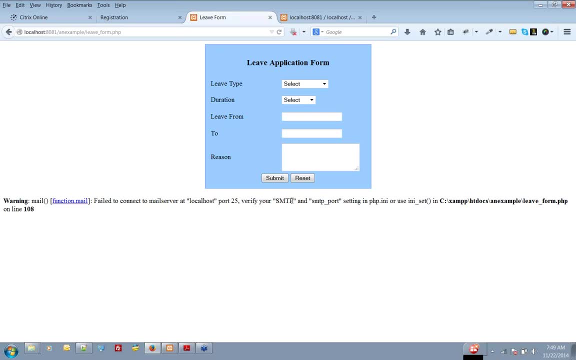 Now we have to use PHP to show and display the errors, Otherwise we can service these kinds of errors. Okay, I'll show you in the code. Okay, So here we are. Okay. So here we are Okay. 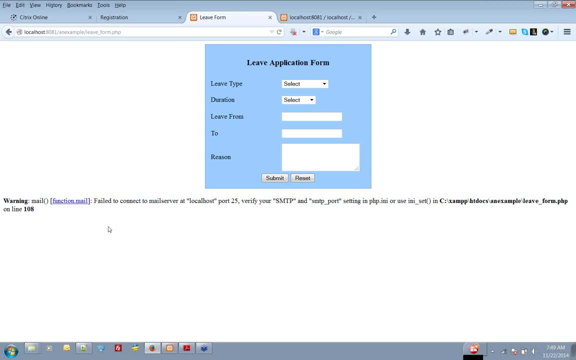 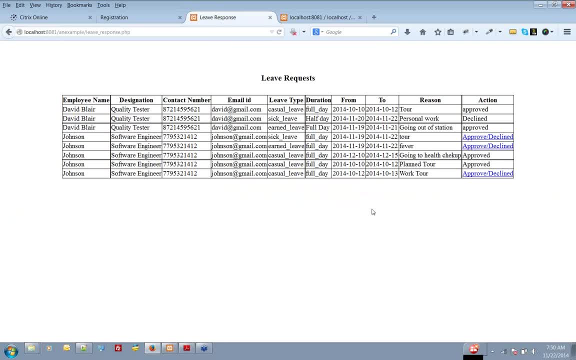 H track restator and this will leave response page where we have received. You can see all the entries coming in. So just now we entered this one. So this column is showing the exact status of the event that we've set. 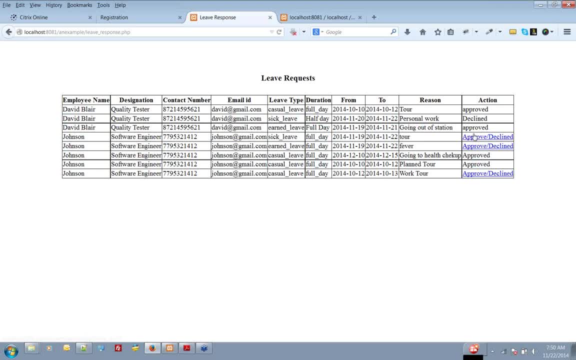 This list is reported. Let's transfer time in this column here. That's it Okay. That's it Okay, Since these are approved. so these we don't have links now take care of this: two links, because this one is approved and this one is rejected. 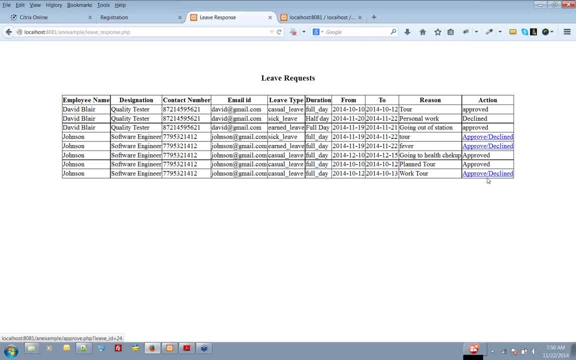 So both have the same parameter, but the function is different. When you approve, look at the URL for this, if you can see this URL, and mouse over is happening on the left corner. So approvepspleavid is equal to 24.. 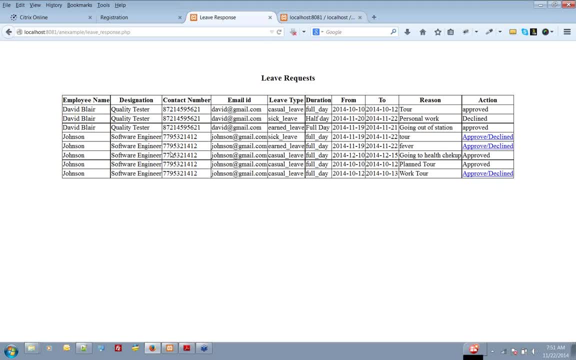 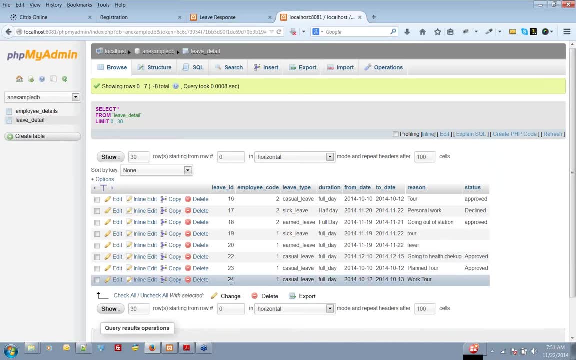 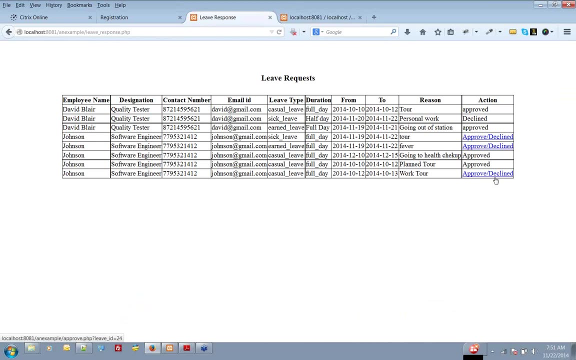 So 24 is the application ID which we have here in leav table. So this one, leavid- the primary key of this table- is 24.. It's shown over here, so leavid is equal to 24.. That means we have to approve or decline the leav request number 24.. 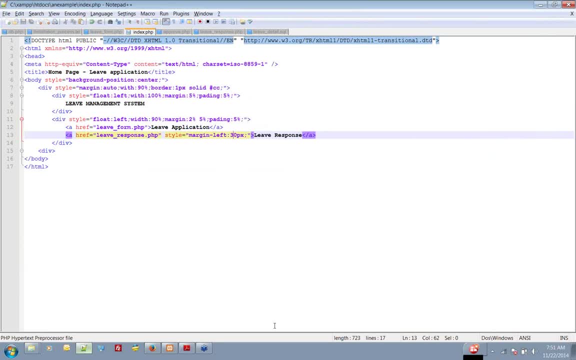 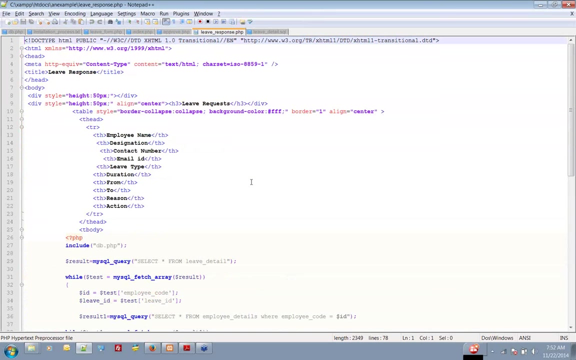 Now let me take you to the code. how it looks like. This is the index page. it has small HTML part. In HTML every document starts with doctype. It has some purpose And the format of HTML. first we'll see leav response. 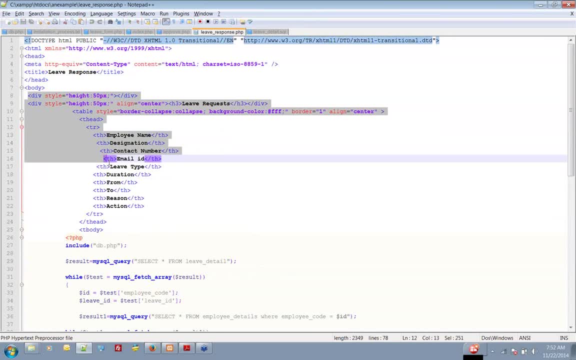 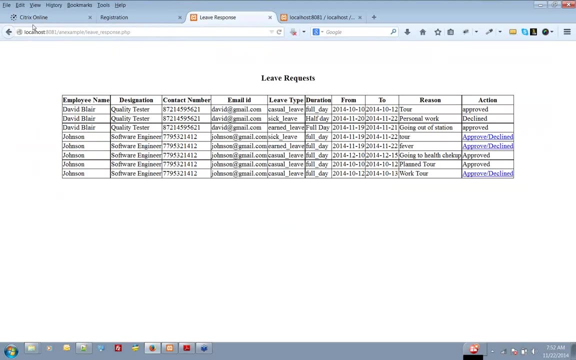 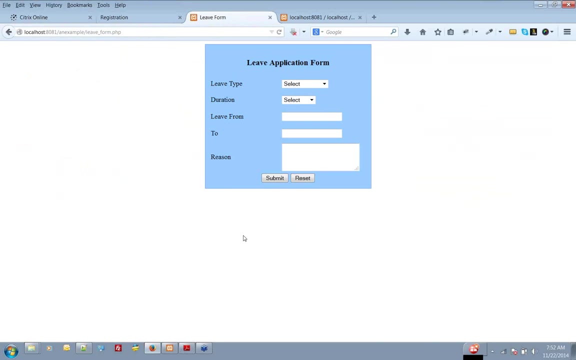 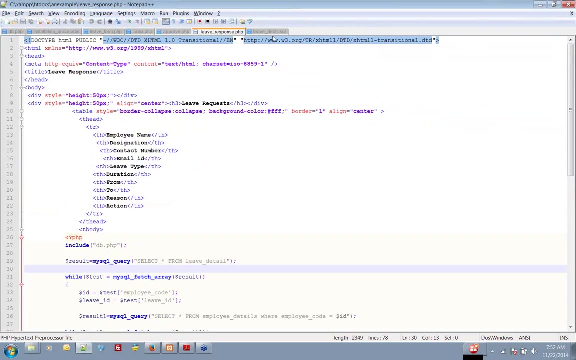 So this is the part which defines your form: leav application form. you must have seen. Let me go back, leav application. So this is leav application form and, under HTML, this is the part. sorry, this one is the leav form. 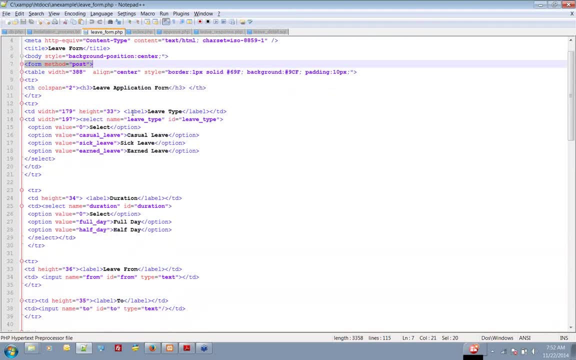 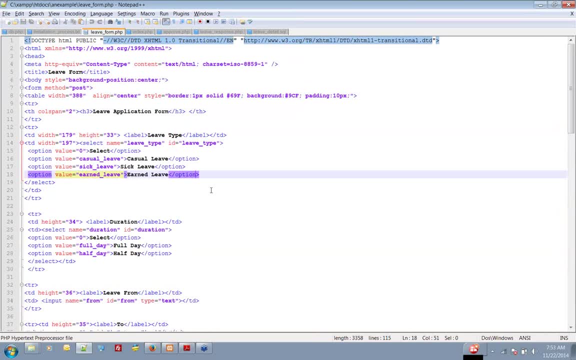 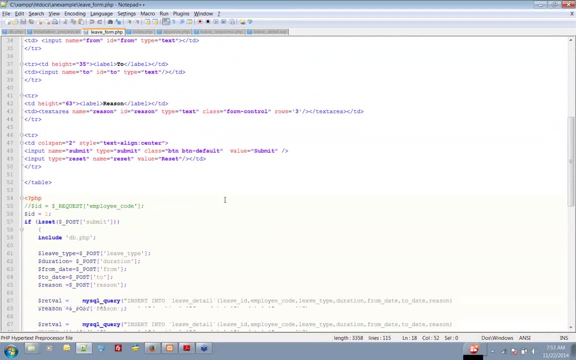 It has a form. Let me go back. OK, I am going to introduce some of my otherlave problems. OK, this one: I am using Notepad++ as the IDE to edit HTML and PHP. For editing the files- PHP files and HTML files- you don't need a particular editor. 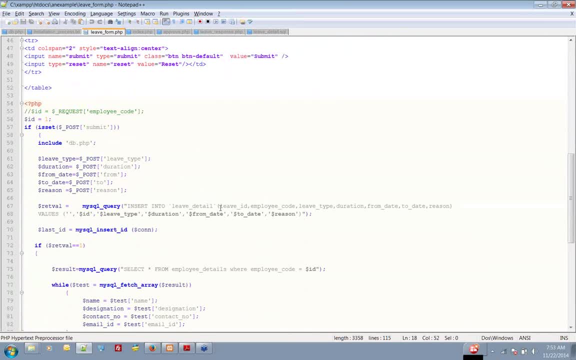 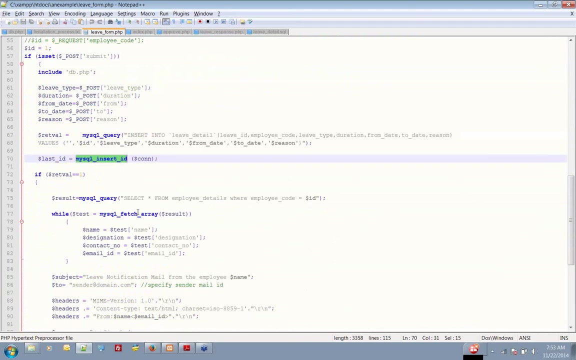 whatever editor you feel comfortable, you can switch to that editor. But if you use zend editor, if you use eclipse, if you use like other editor which comes with PDF, So you will get the help, just like this one. All the keywords, functions will be highlighted in different color. 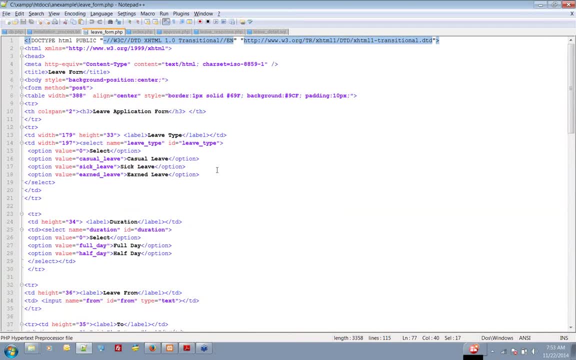 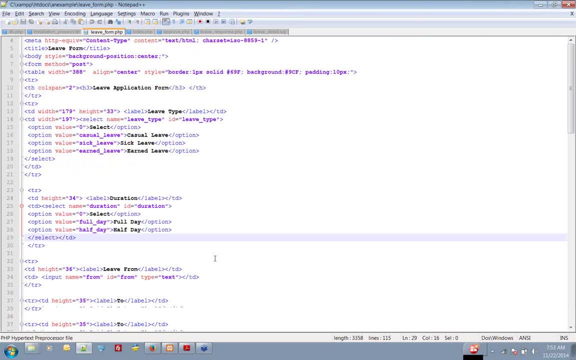 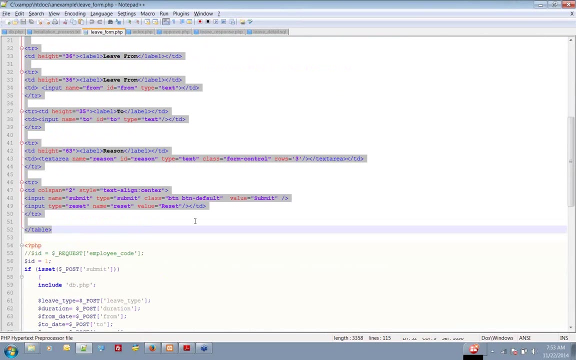 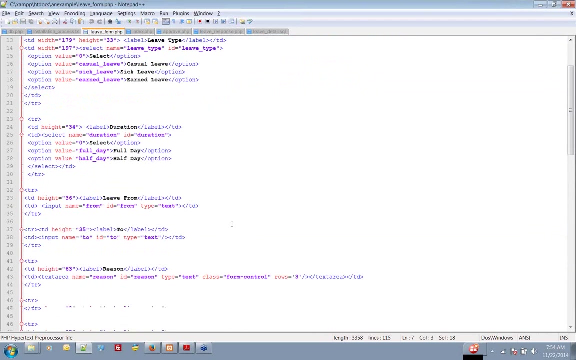 So mostly many editor comes with the plugin nowadays, so you can choose to use any editor. So this is the HTML part where we design the form. Now what will happen once we submit the form? This form, how we can submit, is using submit button. 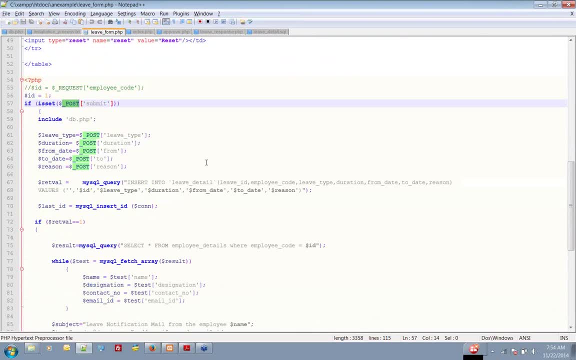 Once we submit. now take a look to this one carefully: dollar underscore post. Dollar underscore post is the PSV variable, which will contain all the data submitted by a form, So this is like a global variable. Submit is the name of this button. 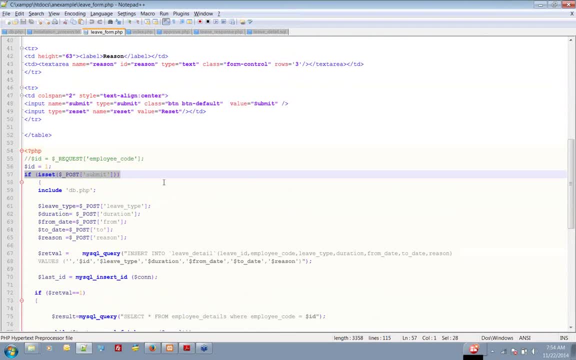 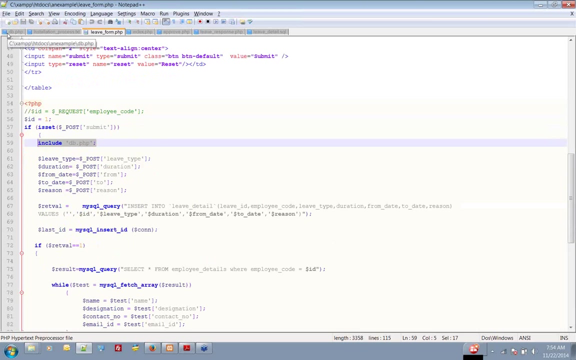 So this statement is to check each set whether the button has been clicked and the form is submitted. So we are taking the condition if the form is submitted, Then we are including a file, dbphp, where we have db related statements. Now this is the line where we are connecting the file. 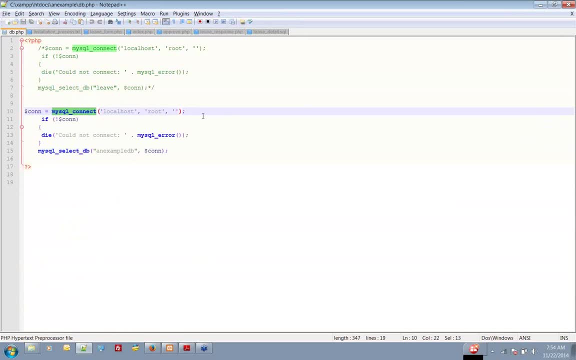 So this is the line where we are connecting the file. I am taking mysql server. I am in mysql, So since this is local host machine, I am using the default username and password. The syntax is like the server name, the username and password. 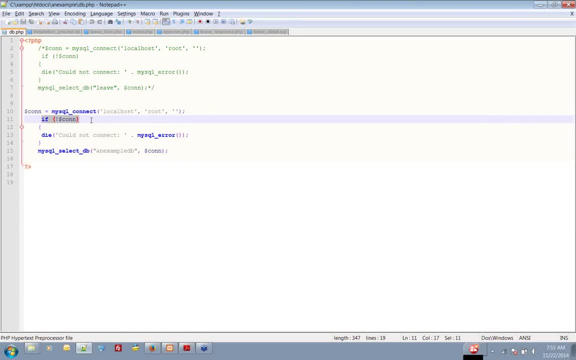 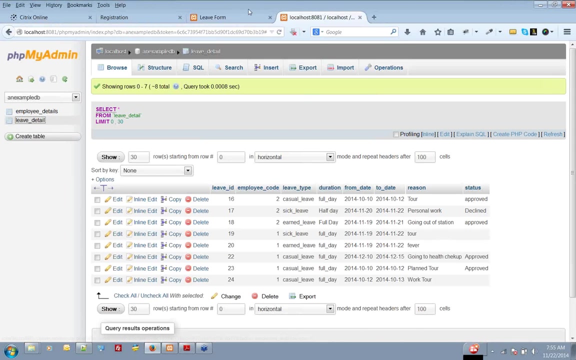 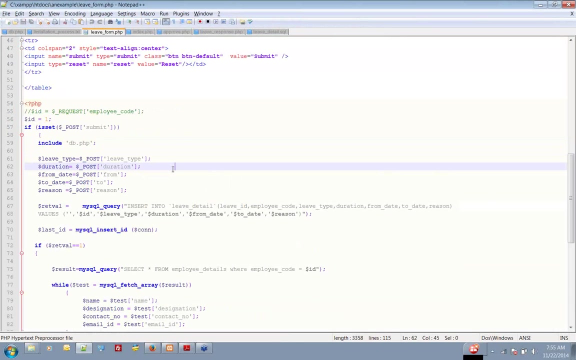 Once you are connected to the server, then select the database. Now this is the database name and example: dbphp. Ok, As you can see, this is the database name. Okay, Now, as I said earlier, include: we have different forms of include. include: include once require. 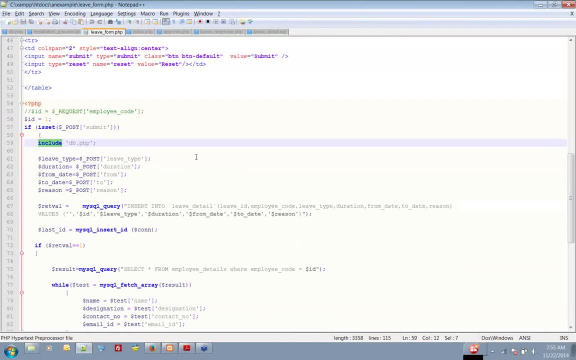 and require once. So there are few differences in all the four functions. Include is like to include the file. include once is to check. suppose there are multiple instances where we need to include the same file to use the same variables. So include once will take care of the fact that the file should be included only once. 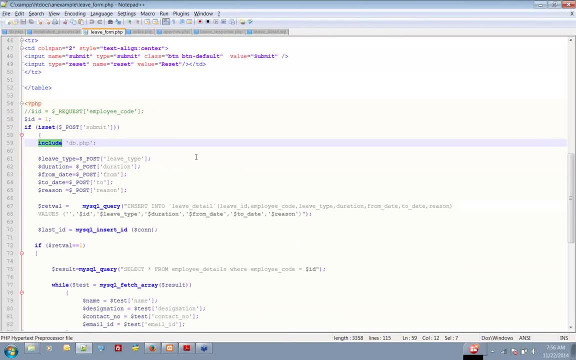 It will not be included again and again. There is one difference into include and require and include once and require once. Include is like Okay, Telling the PHP that I need this file to be included. Require is a strict condition that the script ahead strictly need this file. 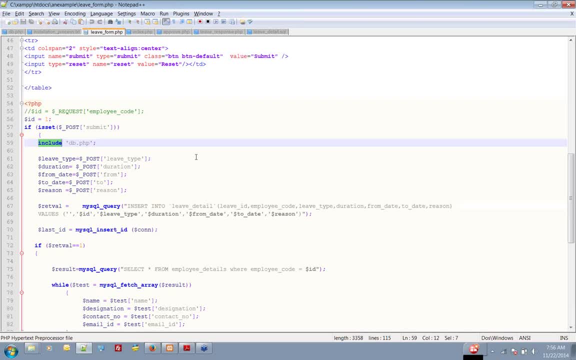 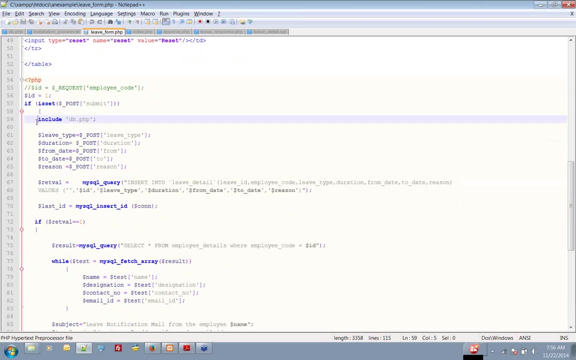 That is the require. Require once is same as include once, But still the require condition is same: It's required. If PHP don't find that file, then it will stop the execution. Okay, Now, after connecting to the database, we are checking all the parameters, which are: 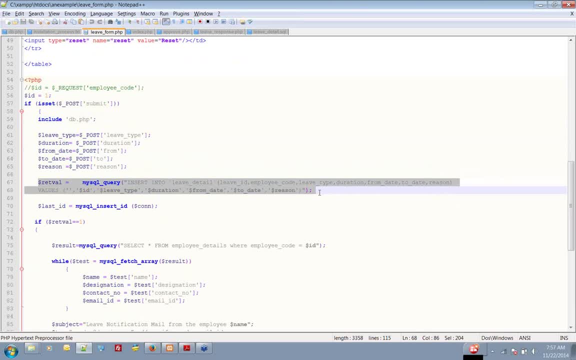 coming from post. This is the query. actual code query. MySQL query. Include leave details. Leave ID is the default field, So we are leaving it primary field, All the other details And we are inserting into leave field. So this is the normal format of a MySQL query. 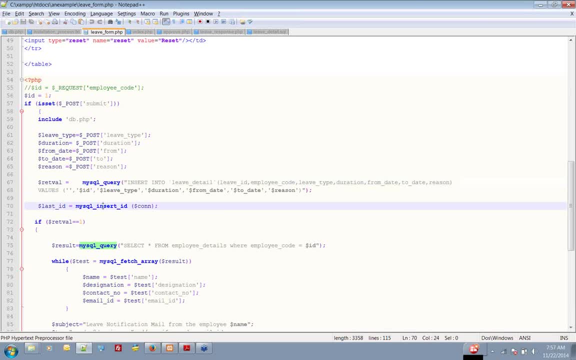 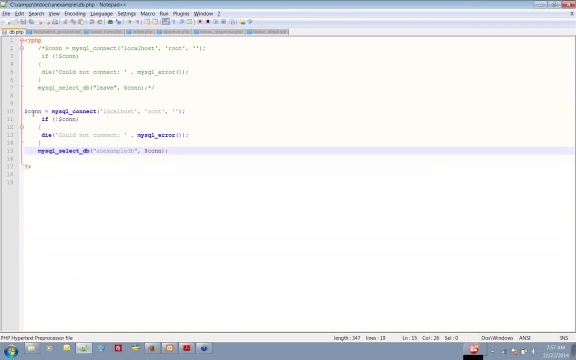 And this function executes this query, MySQL insert ID will be returned. The last insert ID will be returned by this function. MySQL last insert ID, Dollar con is the connection which we have connected here, The con variable here. So we have connected to the server. 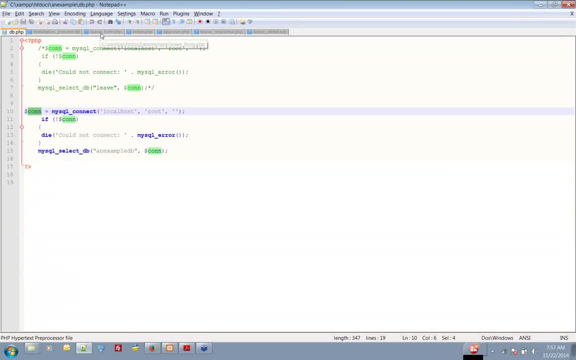 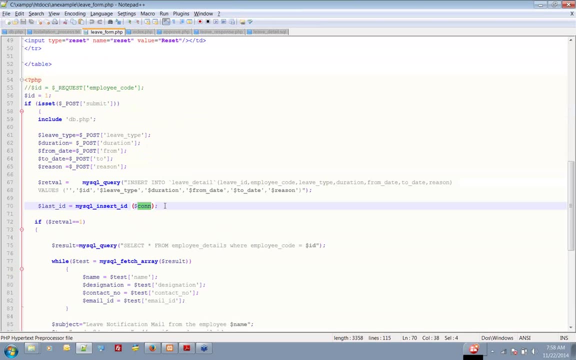 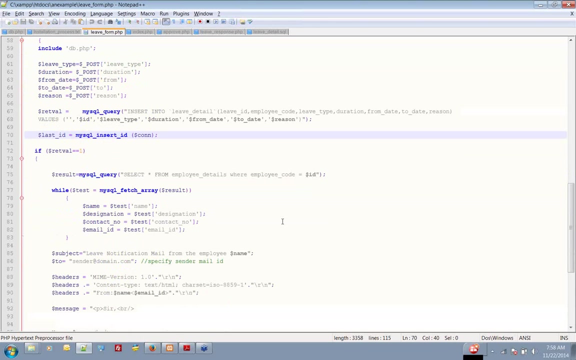 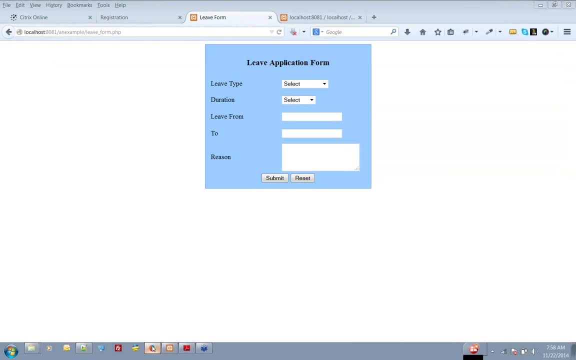 This is the connection string And this, Even if you don't pass, by default it takes the last connected server instance. Similarly, select star from employee. In this example, if you have seen, we are using ID as explicitly one, The employee ID one. 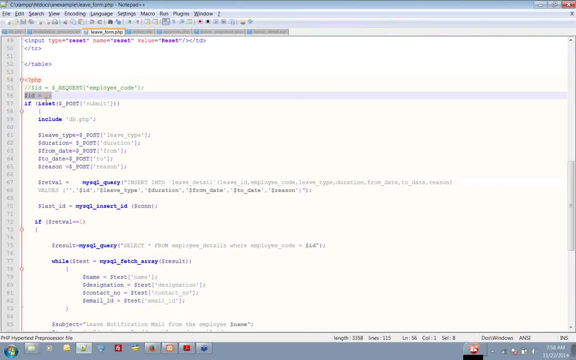 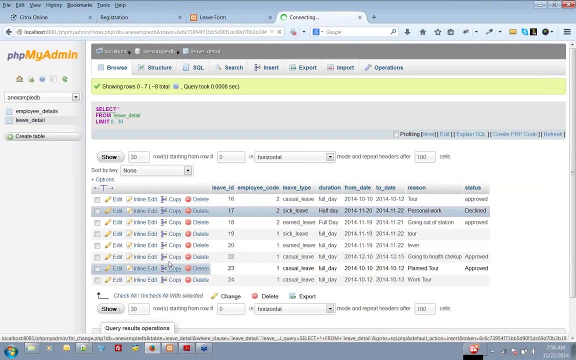 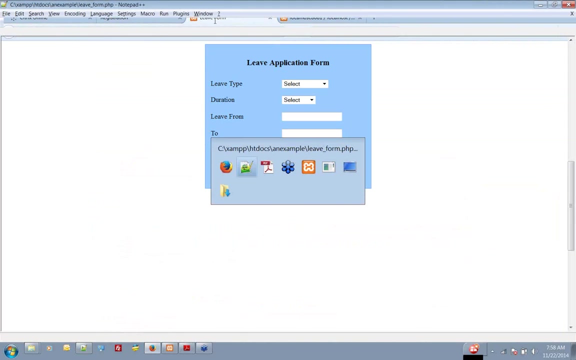 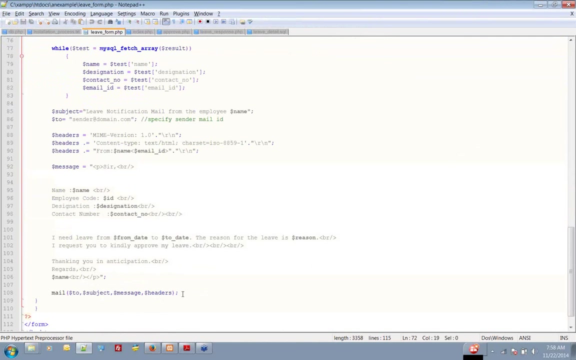 Since we don't have the login form. so what we've done is like we're using static value as employee one. So this is the code And, as I said, mail was not configured Like SMTP. server is not configured On this local machine, so this function is failing. 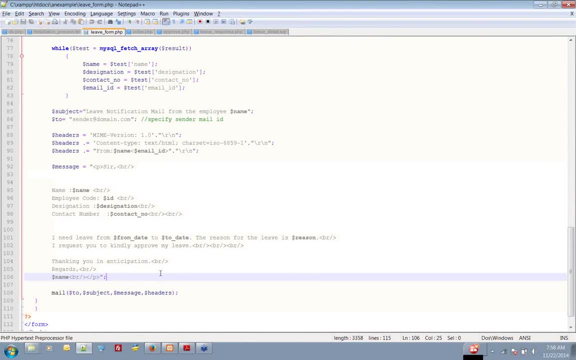 But this is the general structure of a mail, Like how you should be sending mail out of PHP from PHP, So you can set the subject. These are nothing but the variable. now To is the variable. Header is the variable, But this is part of mail headers. 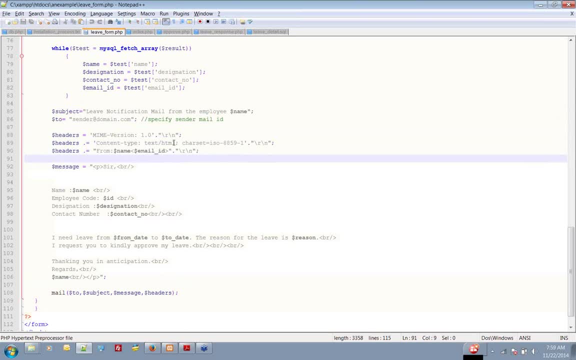 So this is how you define mail header. The content type: text, text email. If you want plain text, that is also possible. Just change this to text or CSV or anything. You can even have the attachment, And this is the body part. 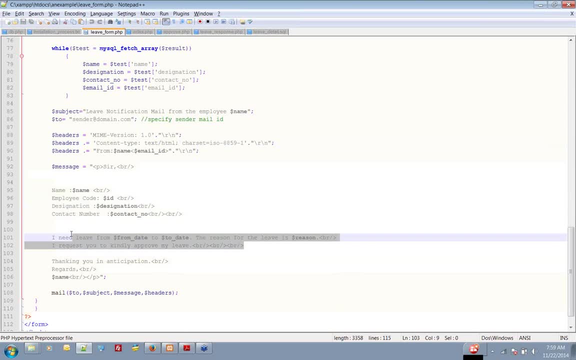 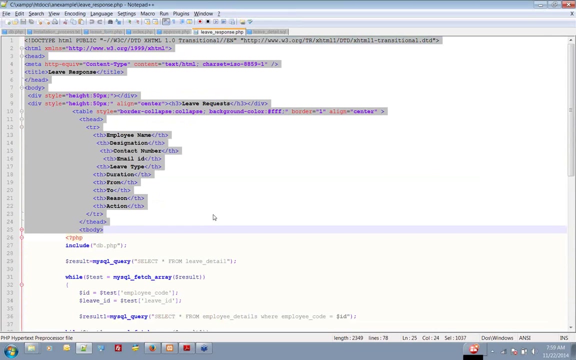 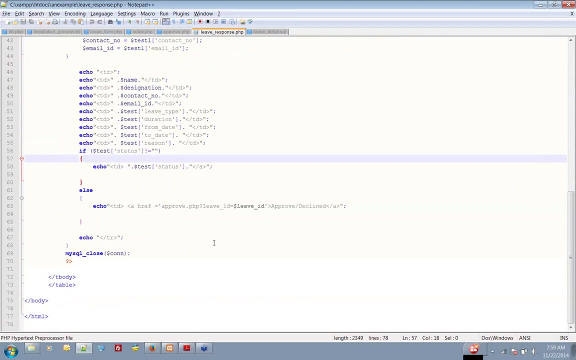 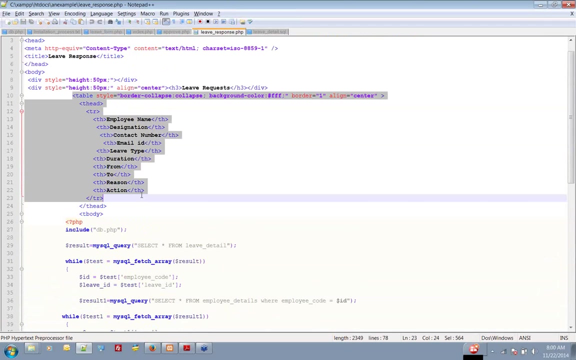 I need leave form. So this is just a message for the administrator to understand your application To notify them On the leave response. we have same HTML part Which will display all the requests. Now take a look to this one. This is the header of the table. 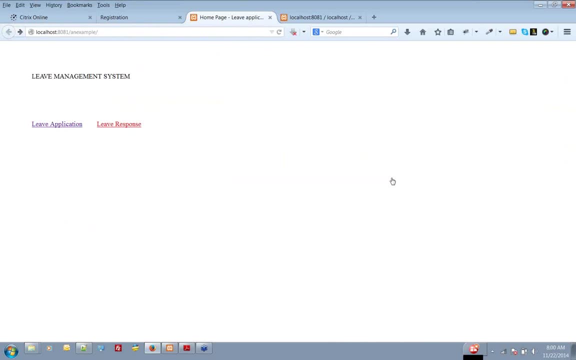 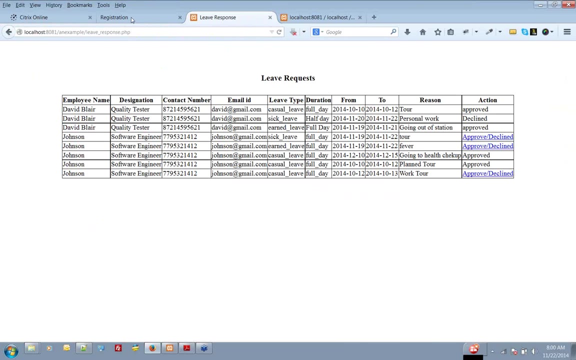 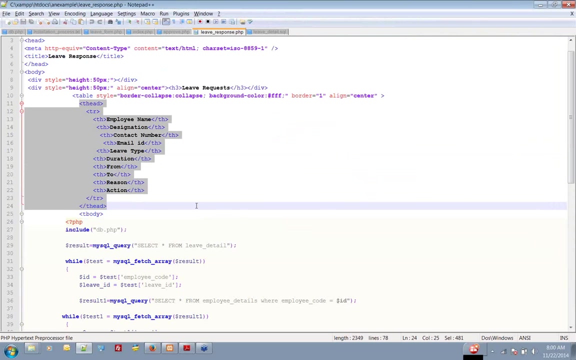 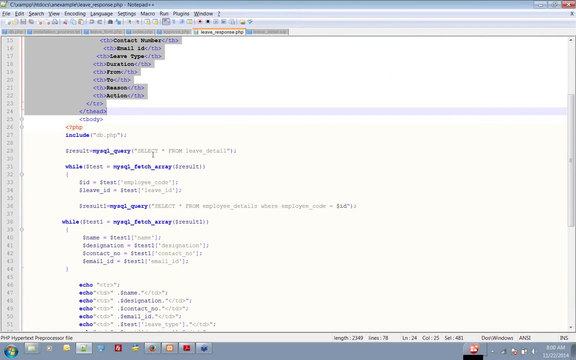 Which is available under leave response. This is table: employee name designation. This is for the HR account. This is the header part. This is the header part: Employee name designation. And the letter part is coming from the database, Which is the data. 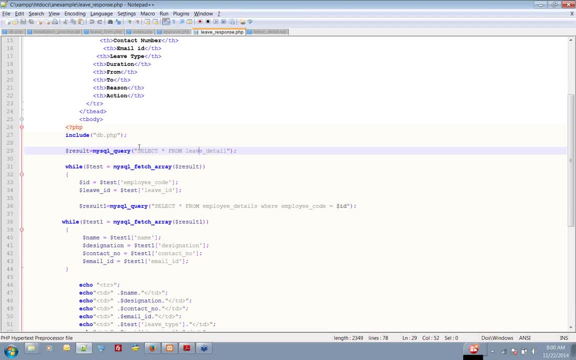 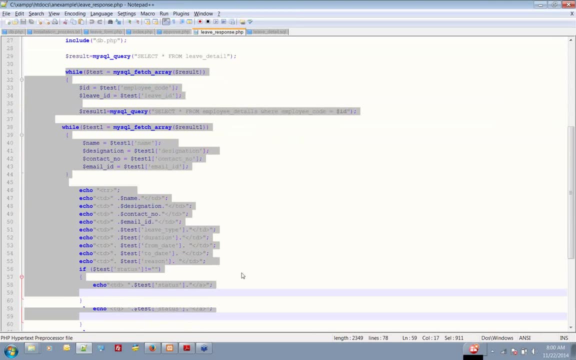 So select. start from the details. All the leaves will be fetched with this query And we are displaying it in a loop. Until and unless you finish displaying all the rows, the loop will continue. Let me just add a little bit of data. 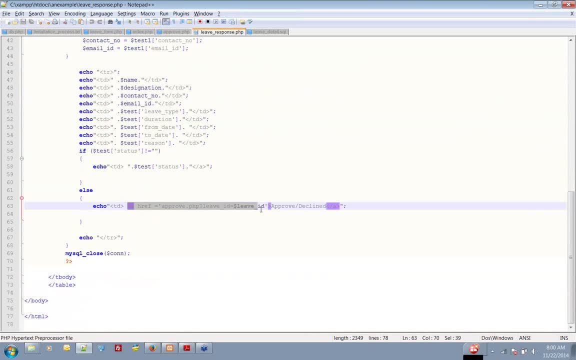 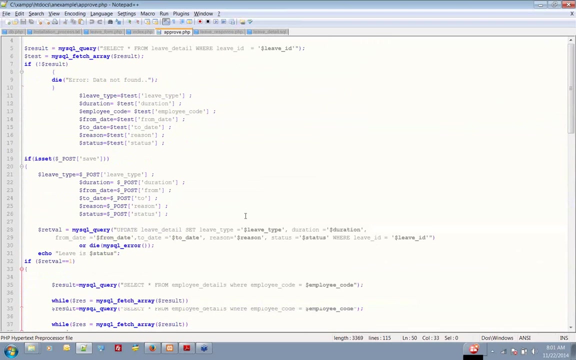 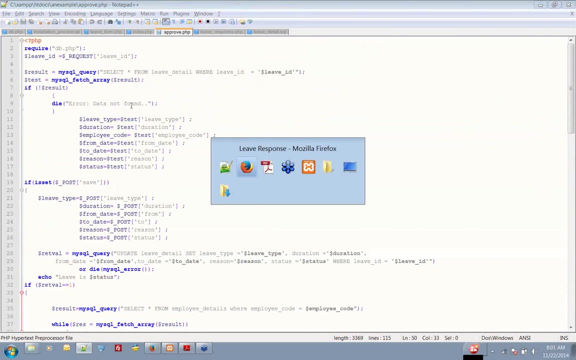 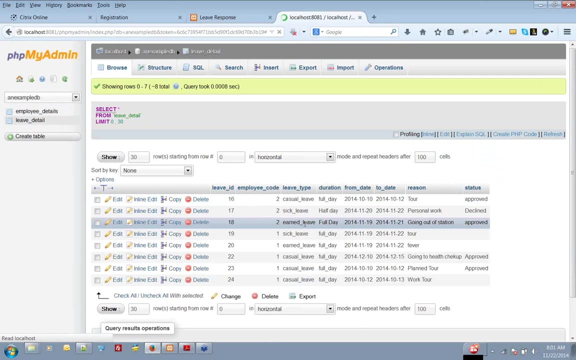 And this is the anchor tag which we will use for the approvephp file. now, in approvephp we have, we have a function which is actually updating one field, this one, this status from live detail table, because the rest every date. everything has come already in this. 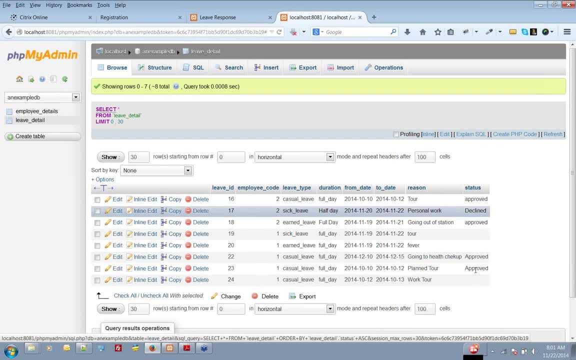 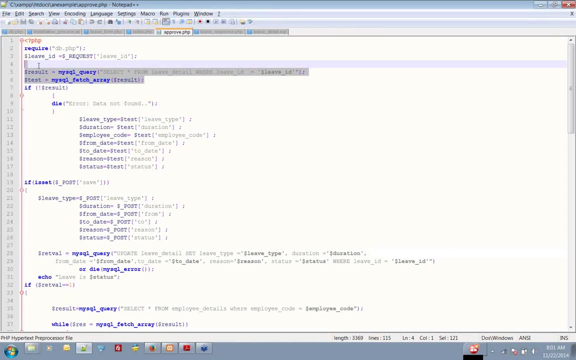 table. So what hr need to update is the status. when the status gets updated, it will be updated automatically. The user or the employee will see whether this leave has been approved or rejected. So we are sending the leave id, which id we need to approve or reject. 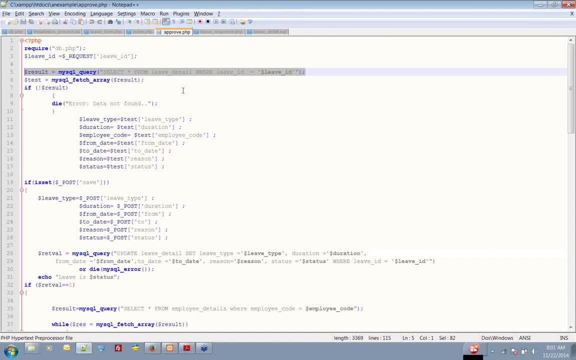 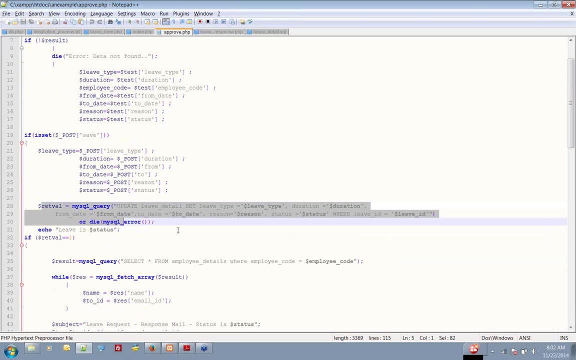 So first, as a normal practice as a developer, we should check whether that leave record is existing or not. If it exists, Then we can- we can go for the update part Here. we are actually updating the status Now. update leave detail. set leave type duration from where leave id is equal to leave id. 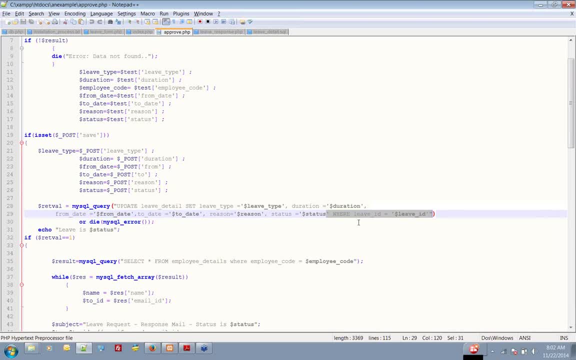 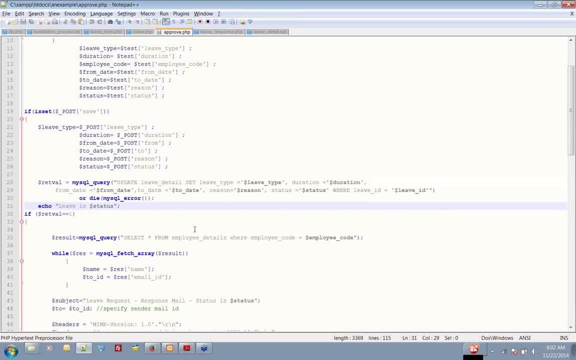 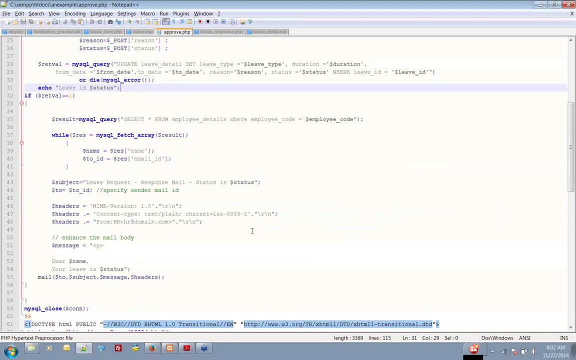 So here is the condition where we find the exact exact leave which we need to update With the status. After that we are displaying Okay. now, in this cycle also, we need to update the employee about his leave: approval or rejection. 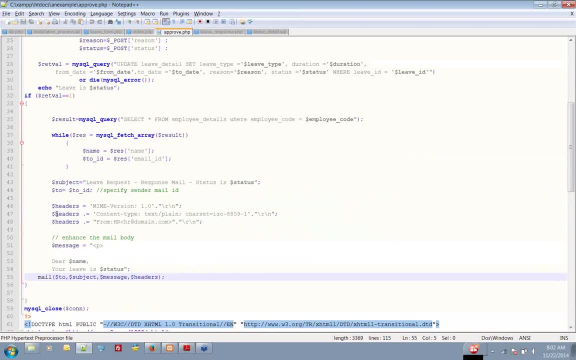 So, again, we are using the same mail function, php mail function, where the subject line will be different, But these are the same variables. Same type of variable. Same type of variable. Okay, Same type of headers. Message will be different. 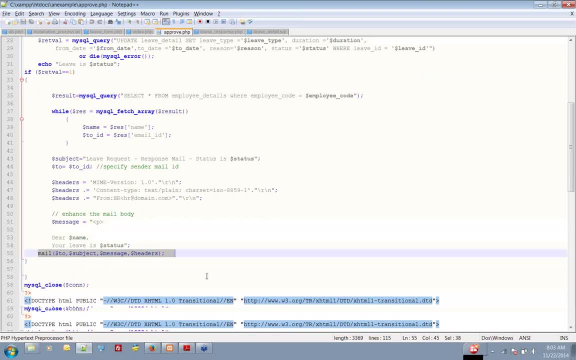 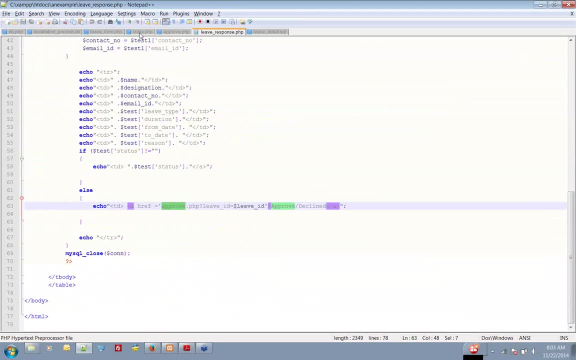 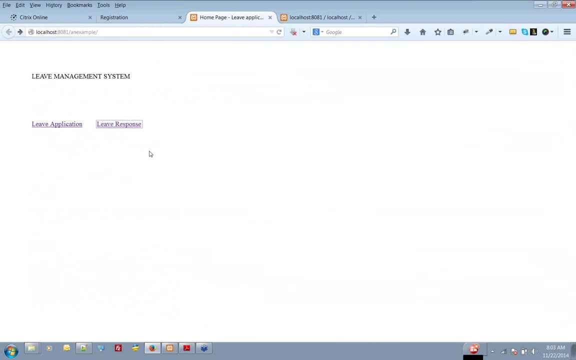 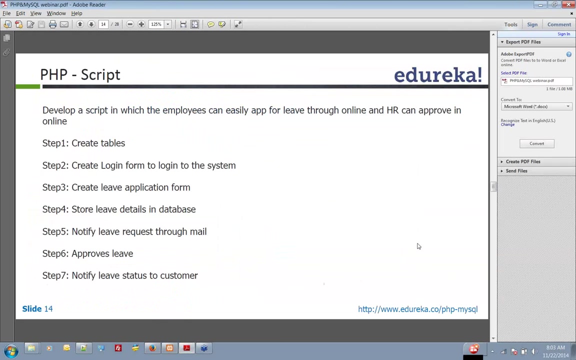 And we are sending it out using mail function. So I hope you must have understood this small application leave management system. It can be a bigger system in the part of the HRMS system. Okay, So what we did, what we actually followed to create this application. 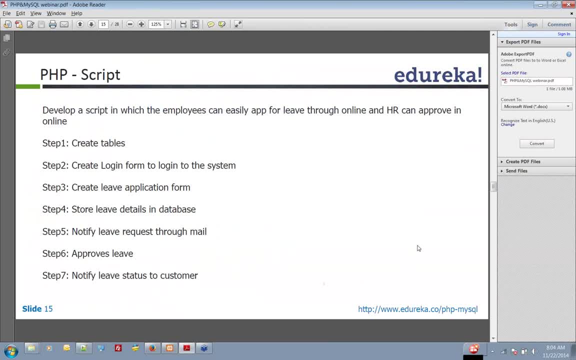 First we need to create the tables, create login form to login to the system. We don't have that login form into this example, but still you can try on your own to have a login information. Sorry, login form where user can login and check his account. 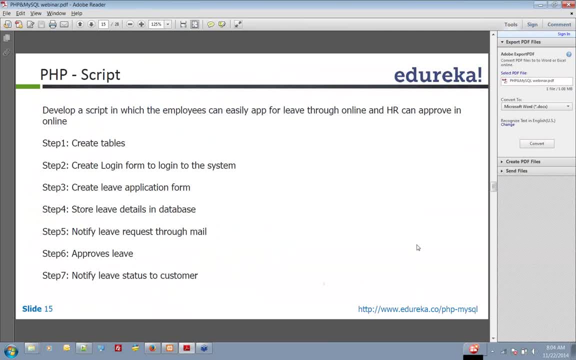 Then we we have a login form. Okay, So in the login form we create leave application form, Store leave details into database, Notify leave request through mail to the HR admin. Or it cannot be just a HR admin, It can be your manager. 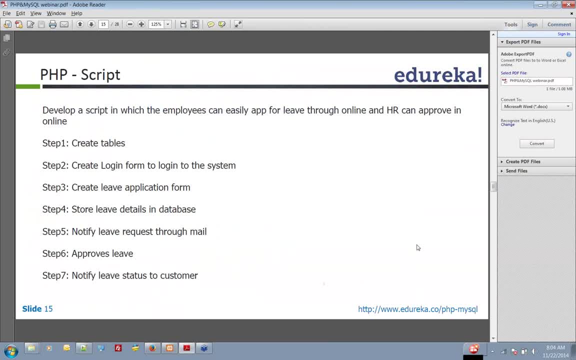 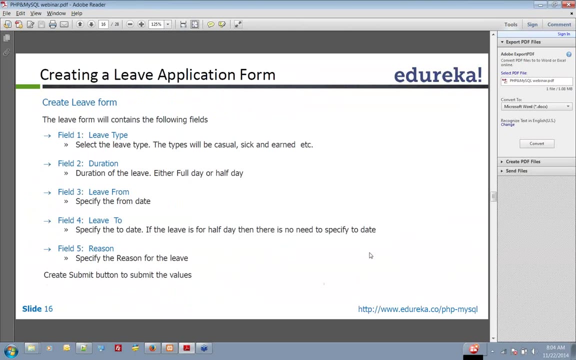 It can be your technology head, So that is dependent on the email address or the database structure it is in. Approves leave customer or the employee. So these are the steps we followed for this application. Now creating a leave application form. So, as I have already shown, the HTML part of the 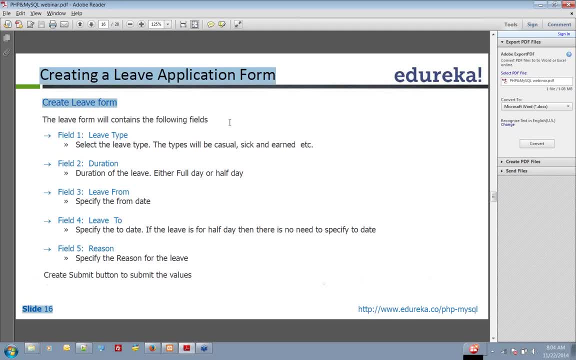 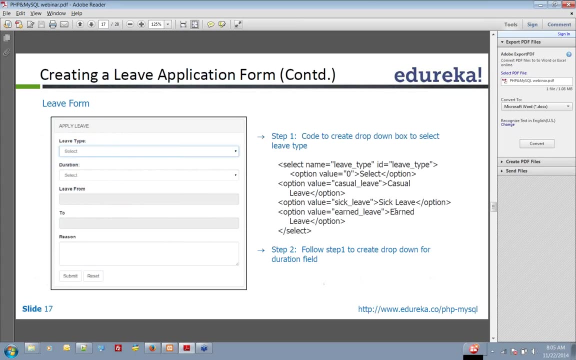 form. So this is nothing but the HTML part explanation where we have leave type, duration, leave form from and to and the region. So these are the values submitted from the form. So this is our form. Now go to create the drop down box to select leave type. So you 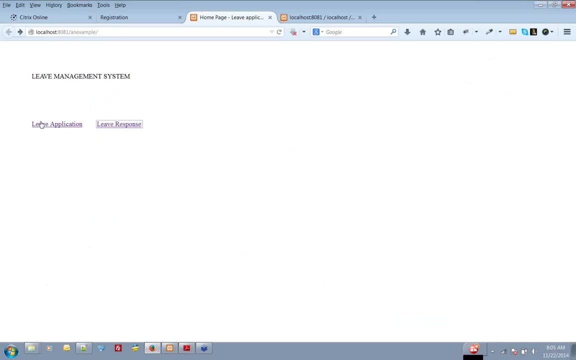 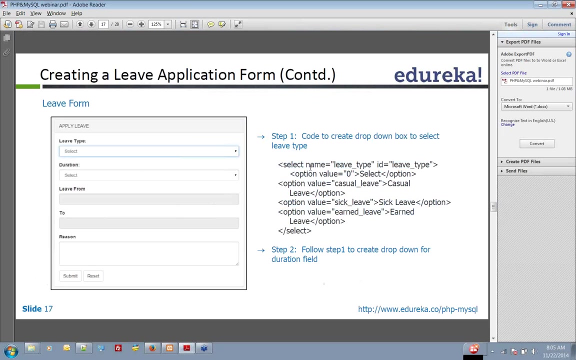 have seen this drop down box in the application page. So this is called a drop down box, where we have multiple values to select So you can select one value from this. So this is the code to create the drop down box: Select name. Name is the name of this element. ID. 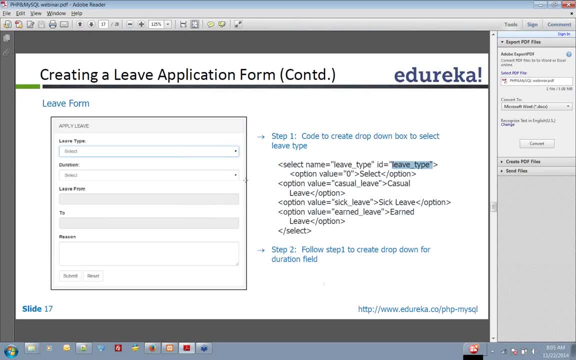 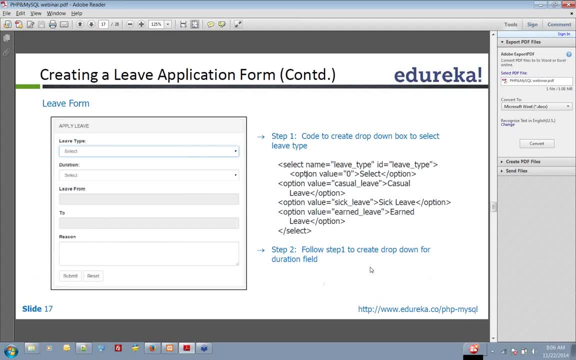 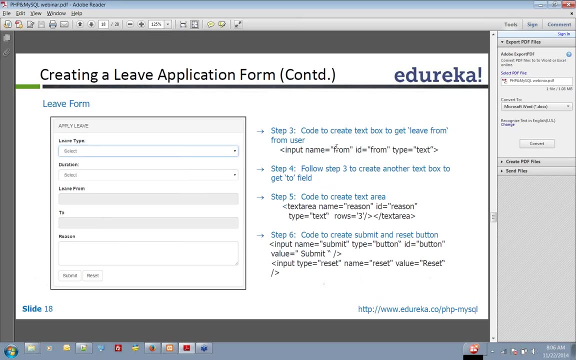 3. And both are as default. Ok for the duration. also same drop down box. You can follow this steps. only Change the name and ID of this element. since this is a different element, Input name from create. Go to create type box to get leave form and leave to So this. 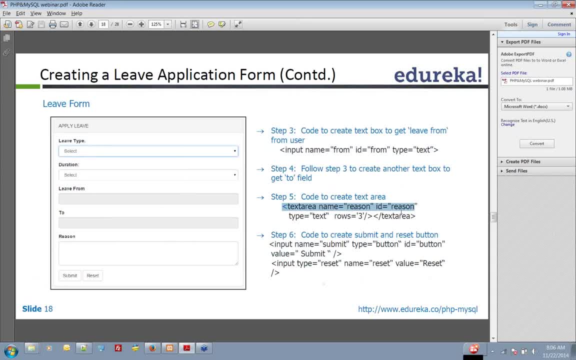 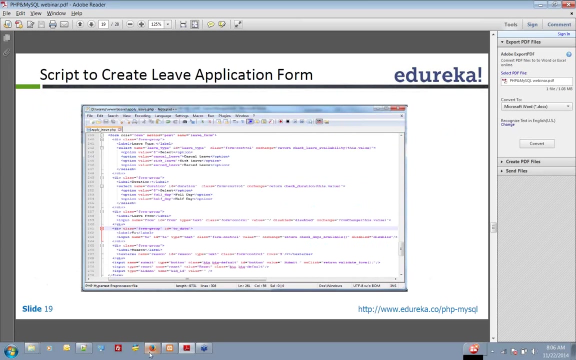 so this is just a normal input type. then textarea to submit the region and the submit button. submit and reset. the main functions of submit is submitting the form. reset will normally reset the form or clear the values. this is the code which we have seen here. the same code. 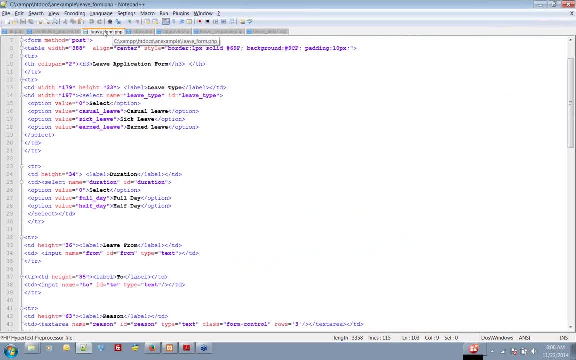 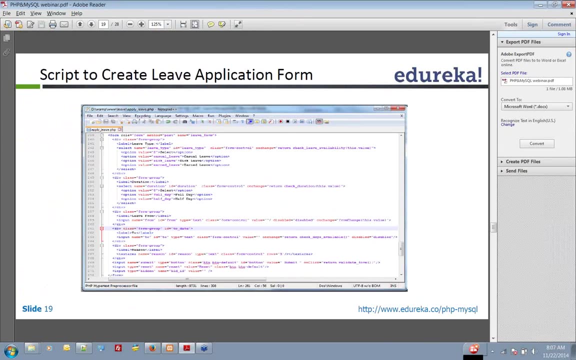 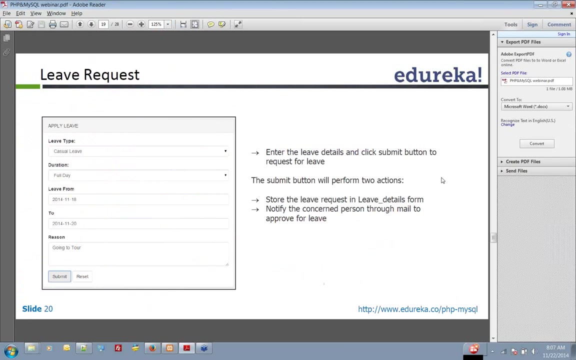 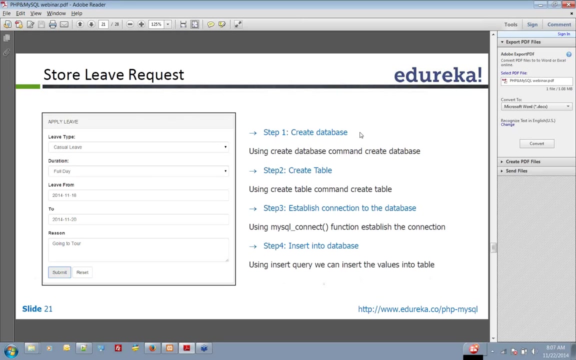 same file. you can choose to have different structure, different names. so here is also in this example we are using notepad++. as I said, id can be used, any id leave request. so normally this is the leave request form with the data storing the leave request. we need the table. 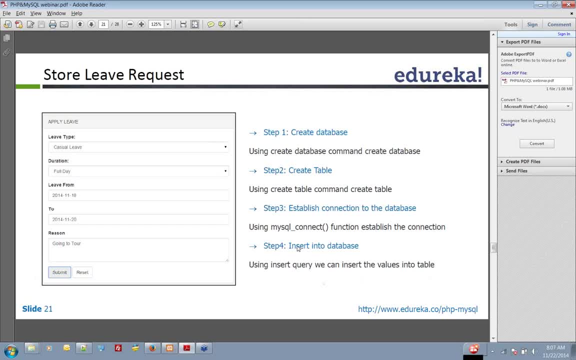 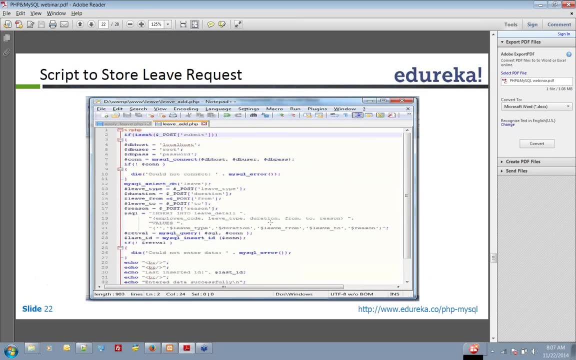 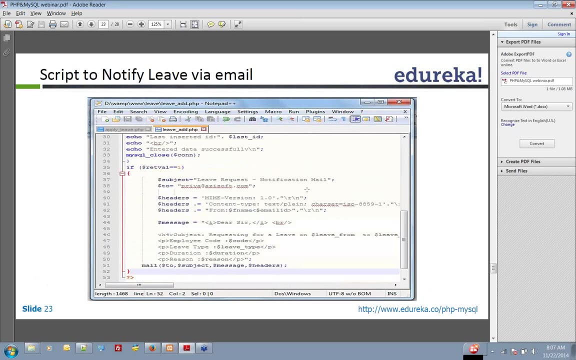 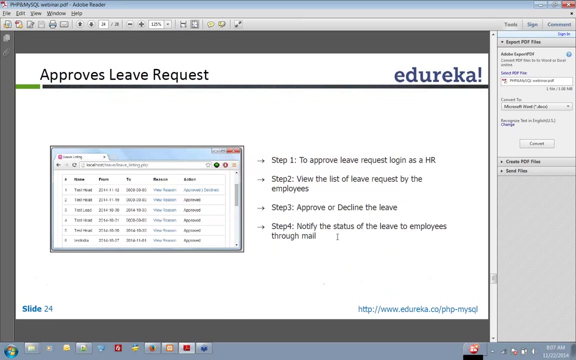 in the database, establish the connection to the database and insert it into the database. so these are the scripts we have already seen: storing and sending the mails out. ok, this is the admin account where admin need to approve or decline, as we have already seen this. to approve: leave request login as hr. 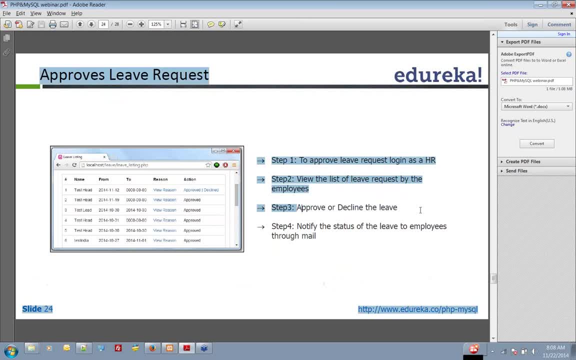 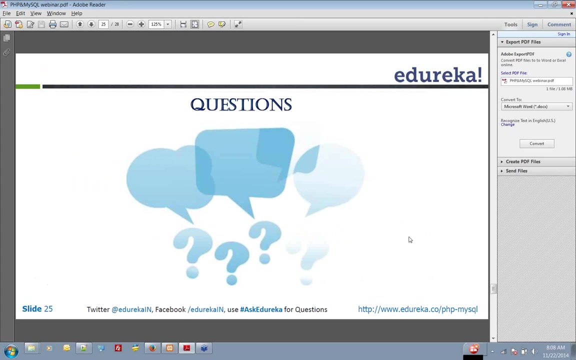 use the list of leave request by employees, approve or decline the leave, notify the status of the leave to employees through mail and notify the client. ok, this is done. now you can ask the questions if you have any. So what Mukul is asking is like why many industries are focusing on Java and NET and there is 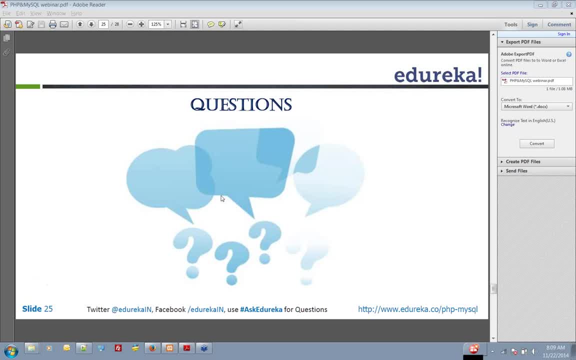 a huge demand for these fields. So actually we have demand in PHP also and like other languages also. Like the nature of Java and NET is a little different and the earlier tradition was to have all the financial applications, all the sensitive information related applications. 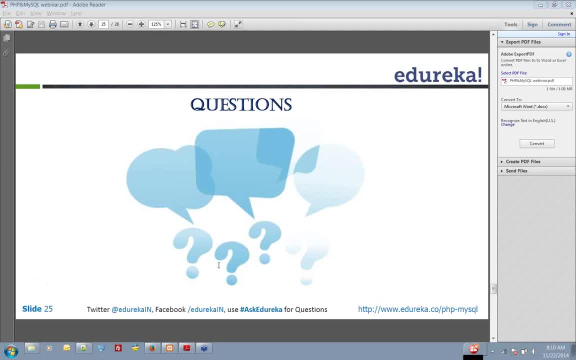 into those languages which are supposed to be more secure. So that is the tradition. It does depend on the programming language, but it depends on the infrastructure as well. So I'm not saying PHP is not that secure. PHP is also that secure. We can make it more secure using the different parameters on the server side in the programming. 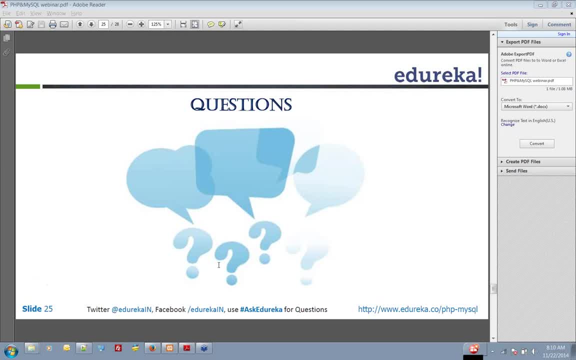 but since Java and NET has all the packages, or it's a complete package of all the libraries, included PHP, since it's an open source, so it has different libraries, even its own libraries, and people also contribute to, you know, to the libraries. 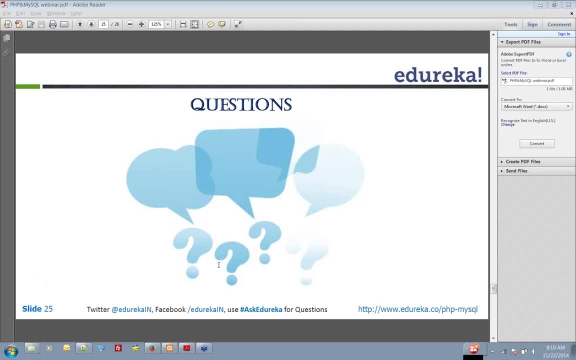 So we can utilize those libraries as well, or you can develop your own libraries to make the application more secure. Okay, Okay, Okay. So let's see. Yes, Mukul, So like since MongoDB- even if you use MongoDB- no SQL, but still you're storing the data- 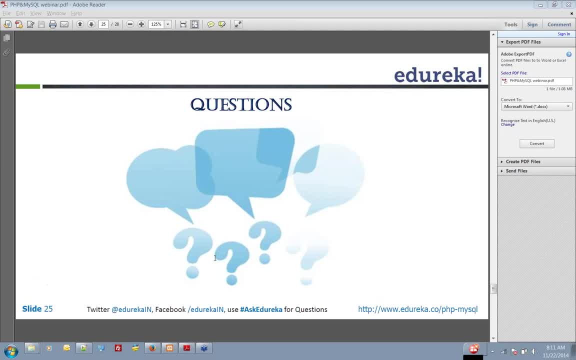 So the chances of SQL injection is not from the database, It's from the form, Because if you're seeing SQL injection attacks, it's like coming in with a database. it's like a database Okay. So let's start the data. 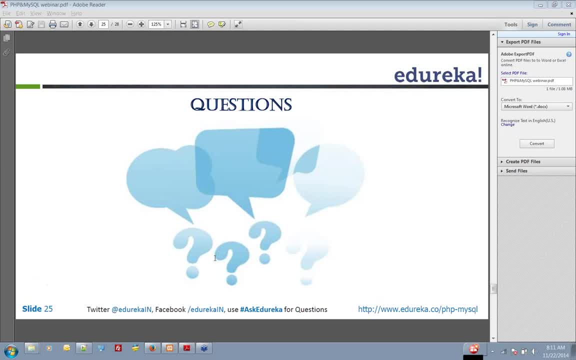 So you still need to take care of executing the queries. It's not only for PHP. even it's happens with other languages also. So everywhere you need to filter out the input data. since you are not like, you have designed the form. So what data is expected by the form? 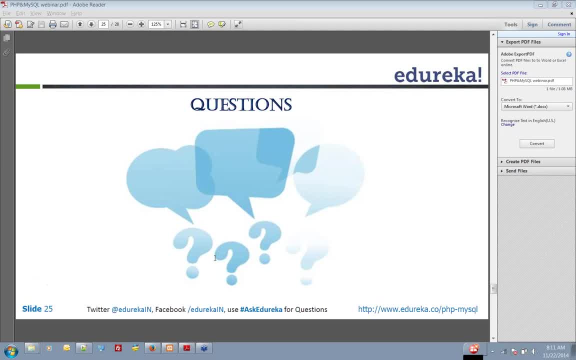 By the each element which we have on the form, So that you need to filter the color. Okay, It's not just SQL commands. What we are passing is like parameters for the input form. So, since we know that it's a database system, so we can have SQL commands which will go along with the data. 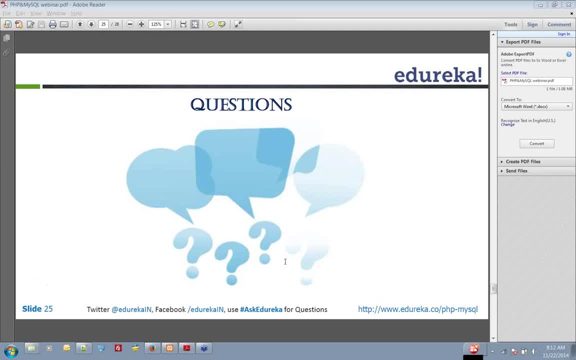 If it is no SQL, if you are a programmer, so you know like what parameters you can use to you know, break the code. So in any case, if you filter the input data, That's a kind of better security for the application. 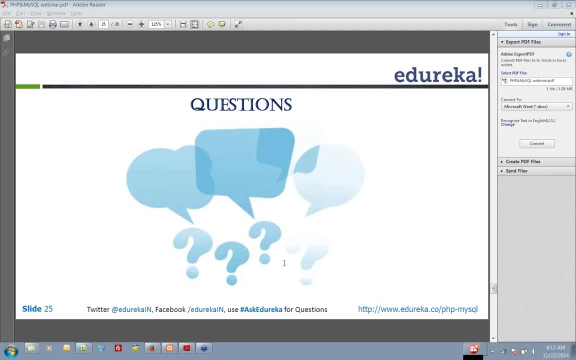 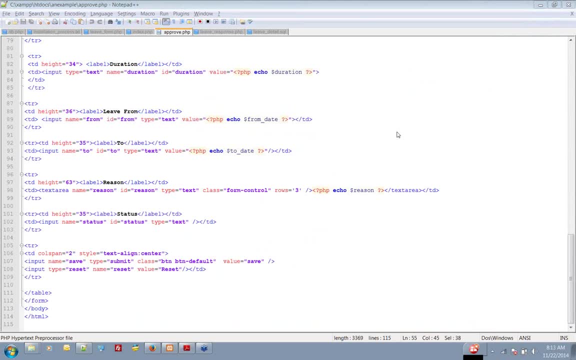 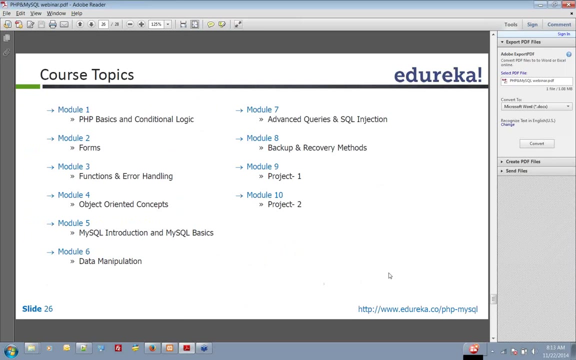 Okay, I guess we are already running late. It's 8.12.. So better go to the next topic. Okay, Now in this PHP course, what? What you'll be learning is PHP basics and conditional logic, how to use control statements, how to use the basics in the, you know, application design or even, if you go for frameworks, how to utilize PHP basics for the frameworks, their forms, functions and error handling. object-oriented concepts. 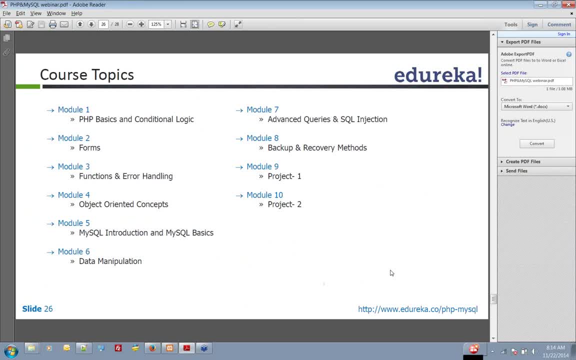 Since PHP supports most of the features of object-oriented. so how to implement object-oriented? Let's see What is the difference. What are the differences? Are the languages of this language. As a programmer, you should keep comparing those, So that will help you to understand the language more. 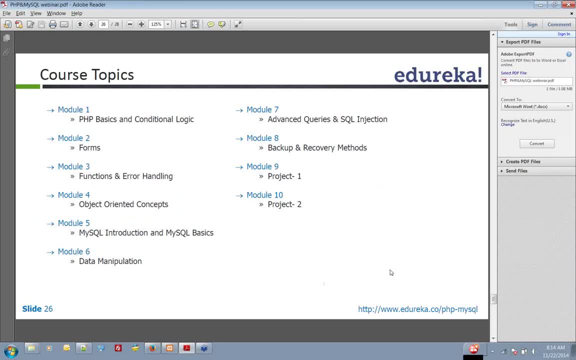 MySQL introduction- MySQL basics: how to. In MySQL introduction you'll be coming across writing MySQL queries, the joins, even running different database tools, like mysql query browser, dpsvimaadmin, which is by default coming up with zap installation data manipulation. 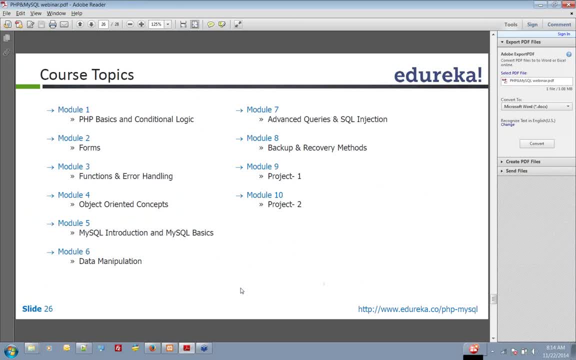 So all these topics will be covered in these models and at the end you will be having two projects. So the one which we have seen is the smaller project, but these two projects at the end will be a complete real time application which you will need to develop on your own. 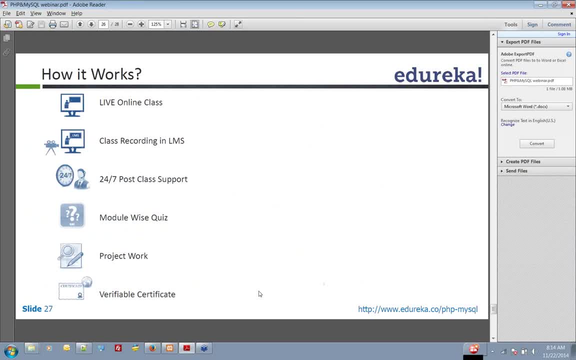 So course will be covering all these things. now, how it works. since it is an online classes, you will have the webinars like this, where our expert will be explaining you all the language details so as they schedule the classes. Class recordings you can find in the LMS. 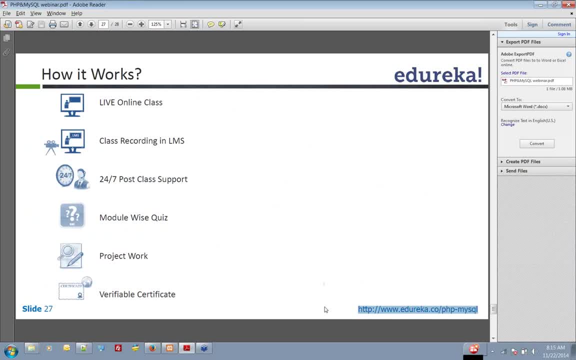 So this is the URL where you can find all the details. you can log in to the system and you can take a look to the recordings. you can listen to the recording anytime You have 24 by 7 post class support where, if you have any questions, any doubts, or if 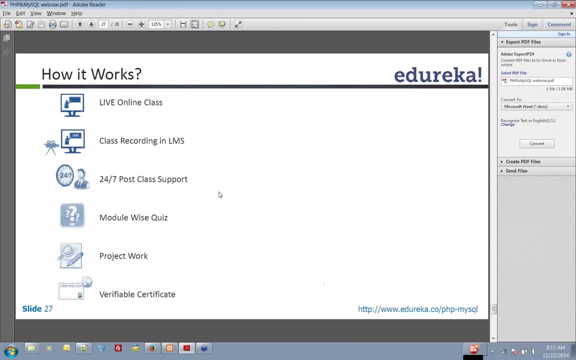 you are trying something and you are stuck anywhere, you can just contact the customer support. So that is it. This is 24 by 7 post class support which you can utilize anytime. Modules will be there so you will be more acquainted with the language, more hands on. 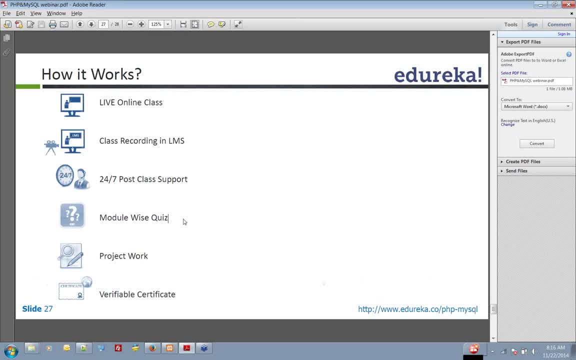 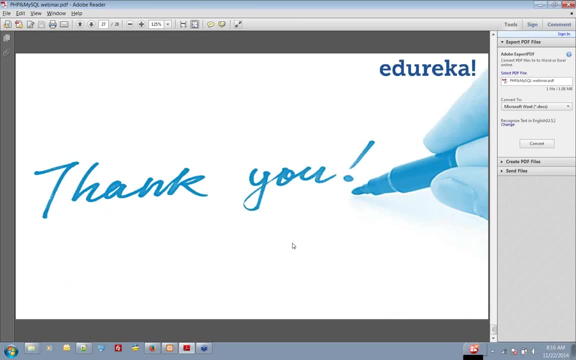 with the technology. the project work is the part of the assignments, and you will have a verifiable certificate which will be recognized by most of the companies. Okay, So I would like to say thank you for attending this session and you can anyway come back. 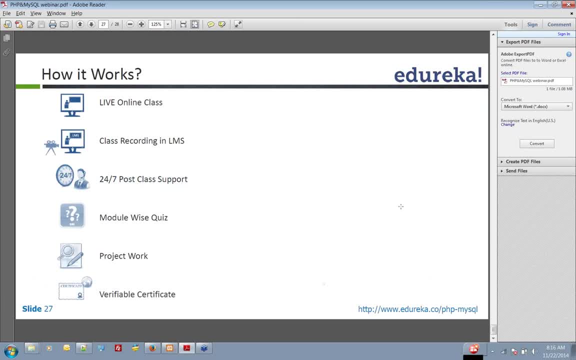 to the support as we have here. So this support or the contact person you can contact anytime for more details, or you can visit the website- this URL on the course details: wwwlmcedu. wwwlmceducom. Thank you, Thank you.